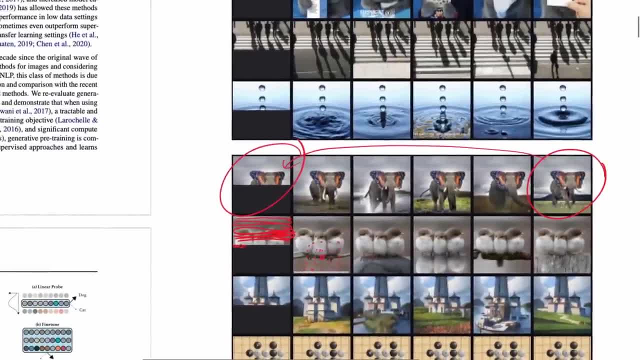 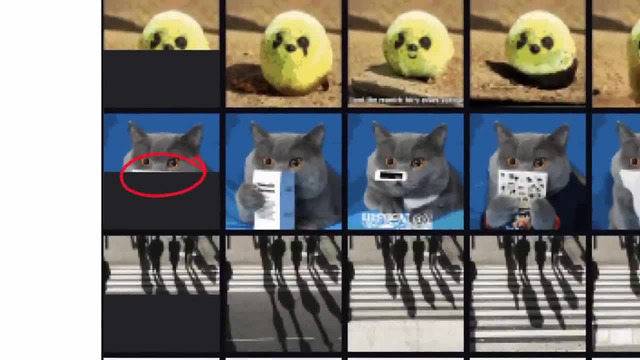 one by one And we'll see how that's done. There are some more examples right here. particularly cool is the cat, And you see that there is the beginning of this little white thing right here, which is this card And the completions of the model. 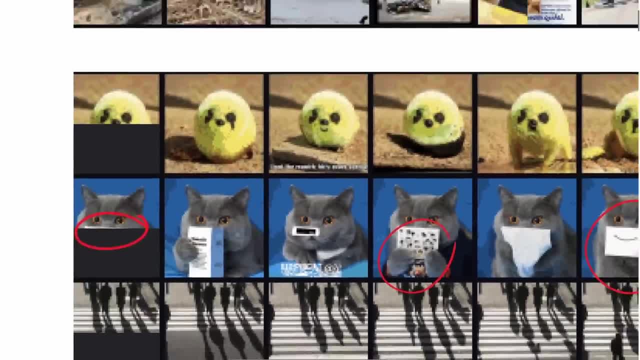 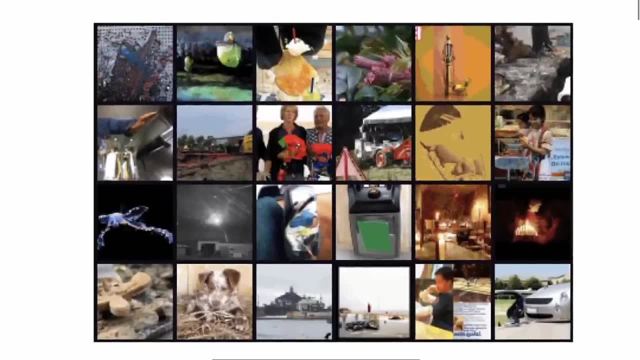 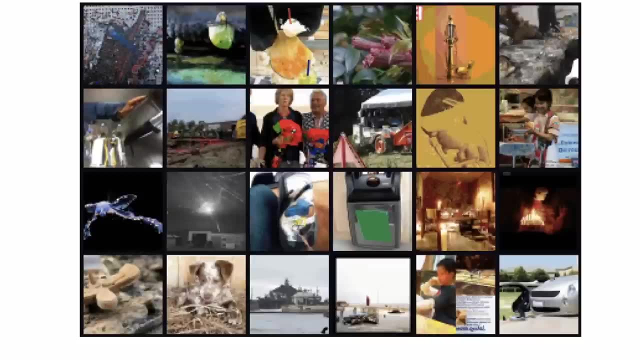 Yes, Very interesting. The model can, of course, as a language model, can also sample by itself just random images. you sample them once through And this is what it comes up with. So these are pretty good quality images for a model that just produces one pixel by one pixel. Now, this idea of 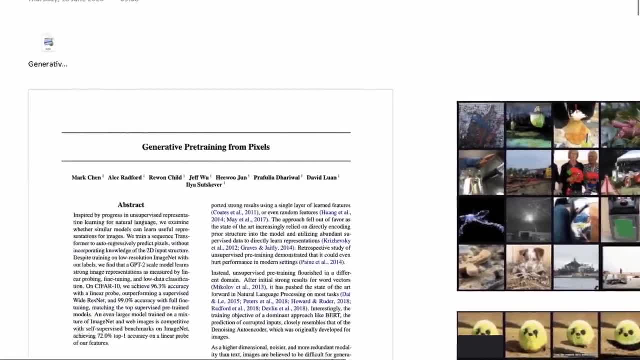 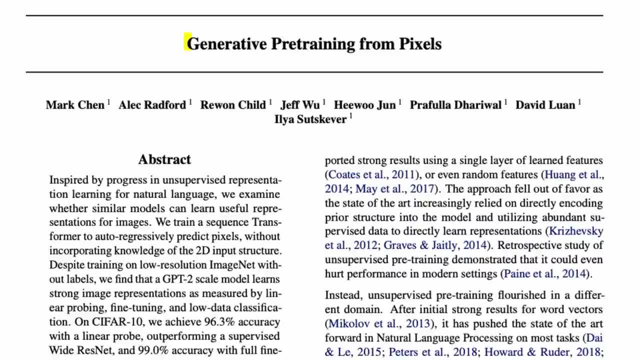 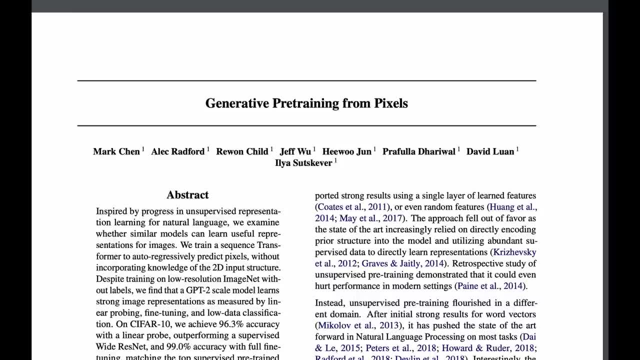 pixel is this And how much pixel is this? And how much pixel is this And how much pixel is this? And can we, how far can we push these generative models for pre training? Yannick Vosghusen. Hi there, this is Yannick from post production. I've realized that I've forgotten. 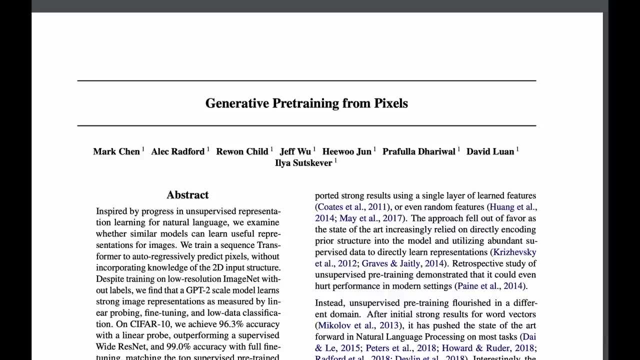 to even read the name of the paper, So it's called Generative pre training from pixels by Marc Chen, Alec Radford, Ravyn Child, Jeff Wu, Hiwun Jhu, Pravala Darywal, David Luan and Ilya Satashkhever, And. 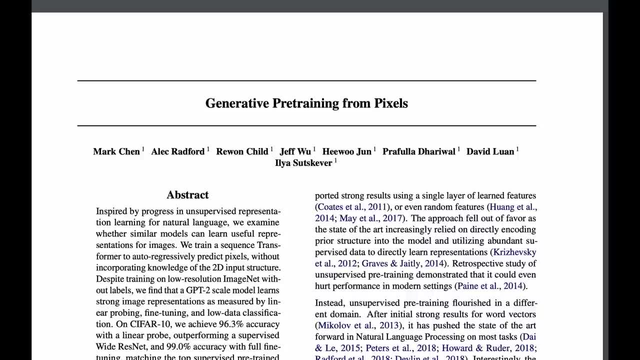 since Henry AI labs has already opened all the models for this course. this is really amazing. Henry AI labs has already made a video on this. This video is going to be more of kind of a rumble rant about what I find interesting about the paper and some thoughts about it, rather than 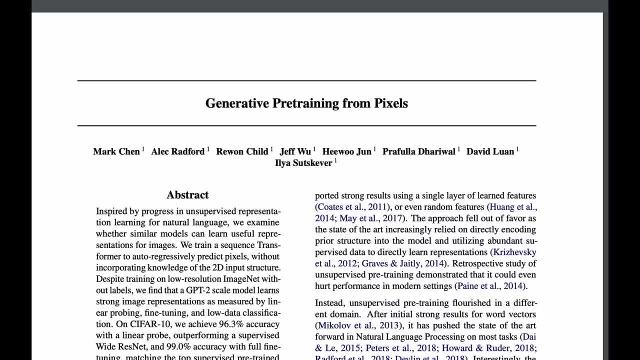 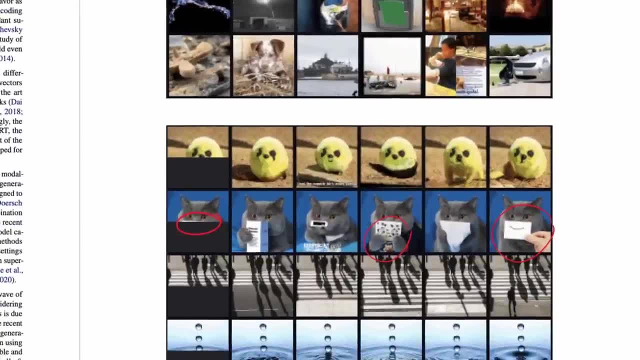 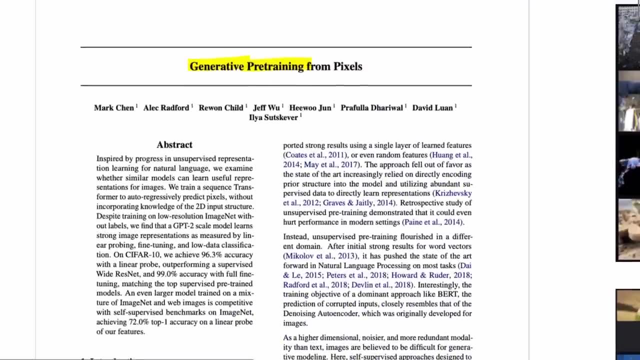 like a classic explanation. I hope you still enjoy that. So what you saw on the right wasn't even the. this isn't the final result, the supposed result. This is simply the pre training task. It's fun to look at it, But the actual object objective of the paper is the following: What if we train? we 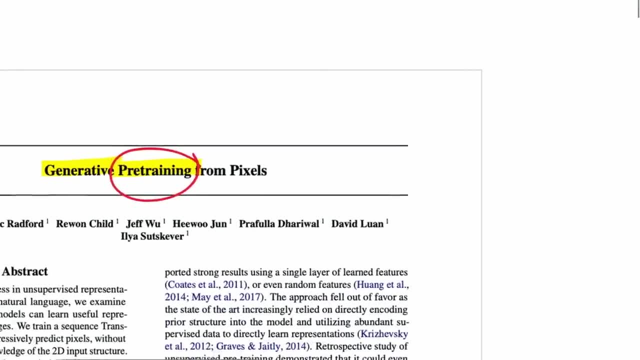 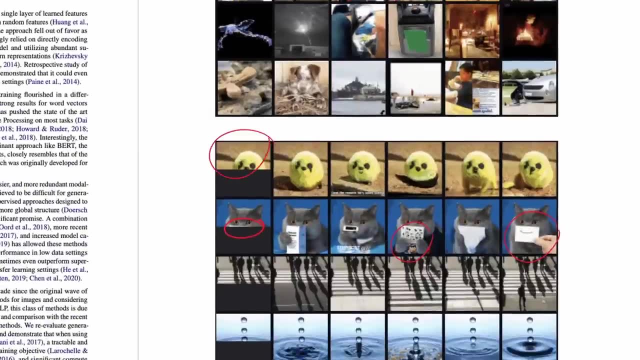 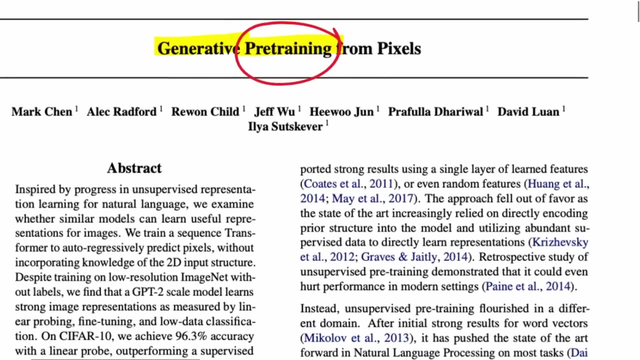 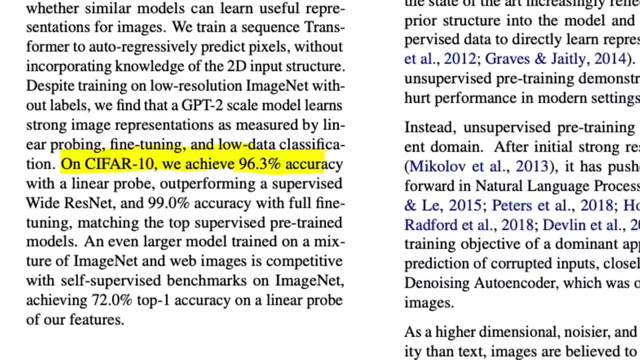 pre train on a large data set to generate what good images like these, or we to complete images like these. And then we fine tune on a classification task And the answer is here. They say: on C2, C3 for 10, we achieve sick the 96.3% accuracy with a linear probe outperforming a super wide. 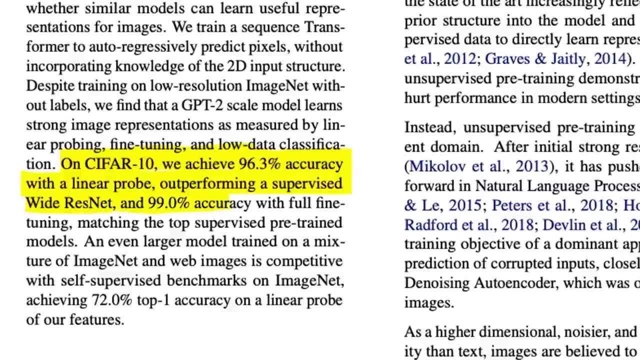 supervised wide resonant and the 99% accuracy with full fine tuning, matching the top supervised pre trained models And even larger model trained on a mixture of image net and web images. is competitive with self supervised benchmarks on image net achieving 72 top one accuracy on a. 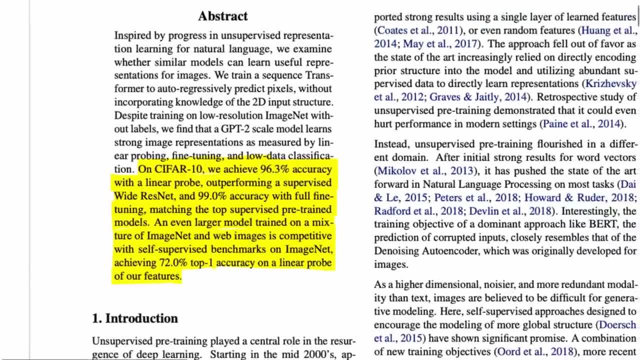 linear probe V2: 4, 8, 5, 7, 8, 10, 10, 13, 14, 23, 24, 25 and 40, 21, 0, 24, 27, 26, 28, 29, 30, 31, 42. 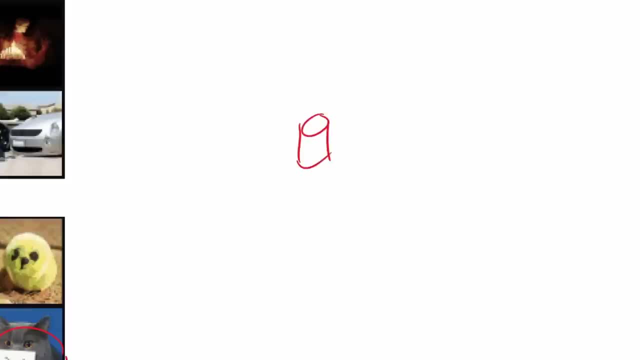 43, 54, 56, 57, 72, 2, 32, 33, 63, 4, 34, 56, 38, 25, 37, 68, 29, 32, 32, 32, 34, 36, 24, 32, 34, 35. 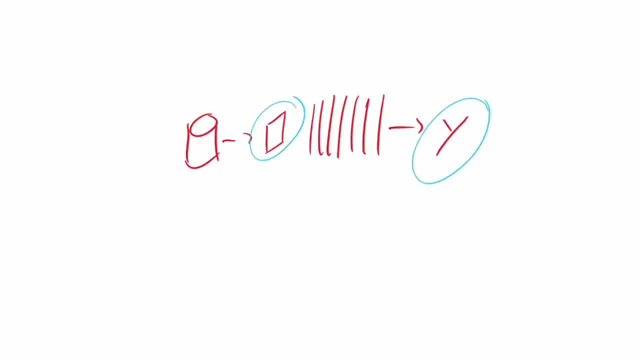 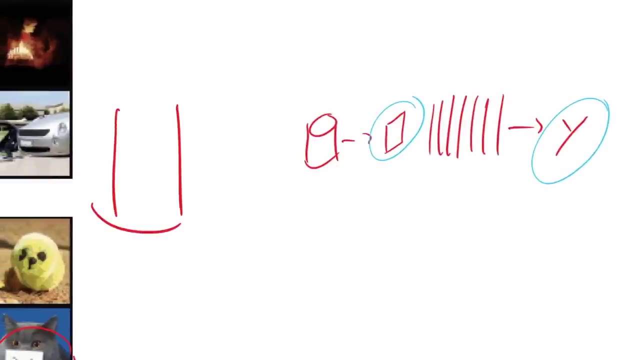 36, 36, 36, 37, 37, crisis, 37, 38? is these images together with these labels? Now, the idea of pre training is that you somewhere have a bigger data set that is sort of similar to the small data set, But, yeah, it's similar enough. 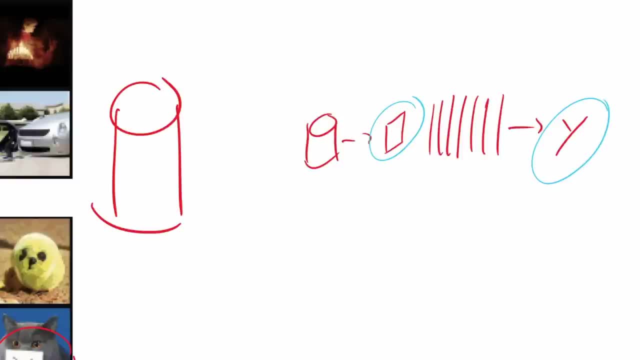 such that the network could learn something. So what you want to do first is you first want to take the large data set, train this network right here, And then, in a second step, fine tune the network on this smaller data set And you sort of hope that what you learned from the large data set 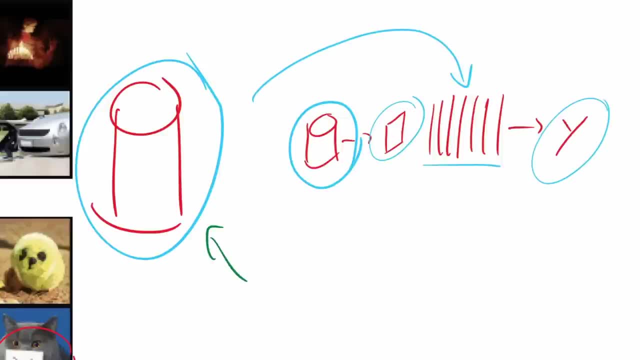 right here transfers over a little bit of knowledge. you already have a little bit of knowledge and you can make better use of the data that you have right here. Now the question is: how do you do this? pre training, And, of course, this has a long tradition- well long for maybe. 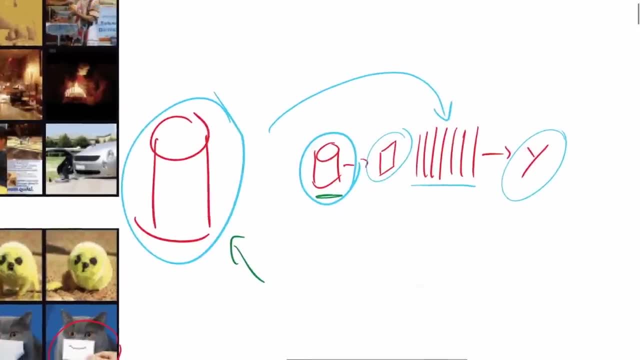 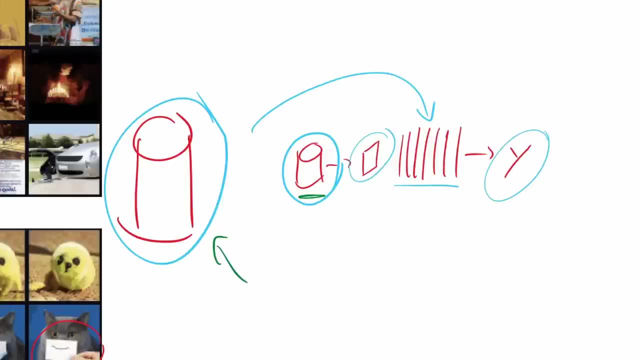 two or three years right now in the language community, where people they pre train these large data sets and then they can make better use of the data that they have right here. models like we've just seen- GPT three or BERT was one of them- They pre train these large 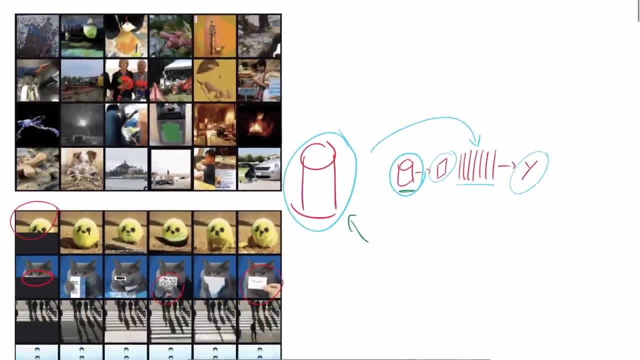 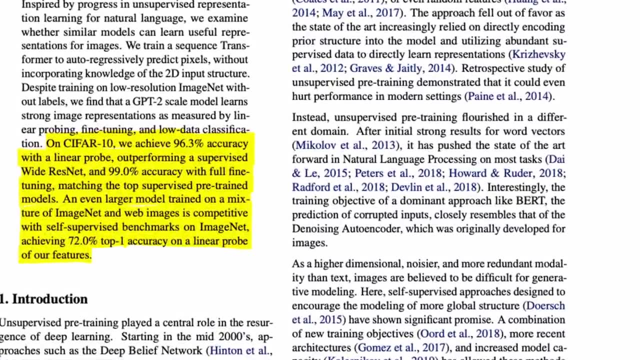 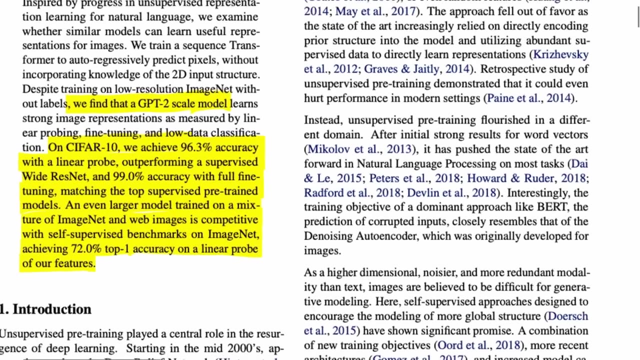 transformer models on text and then to fine tune them on classification tasks for text. And that's what this paper is doing right here. They pre train a transformer, that is a GPT two scale model, They pre train it on image generation And then they fine tune it. or 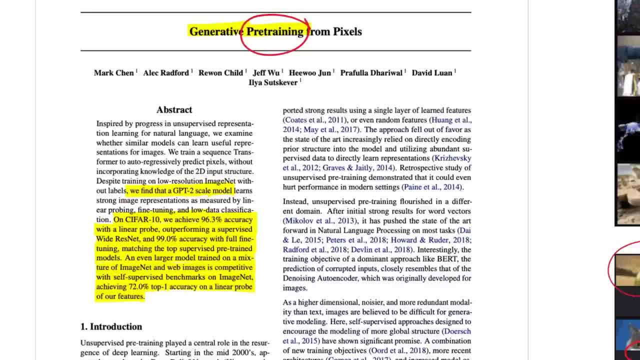 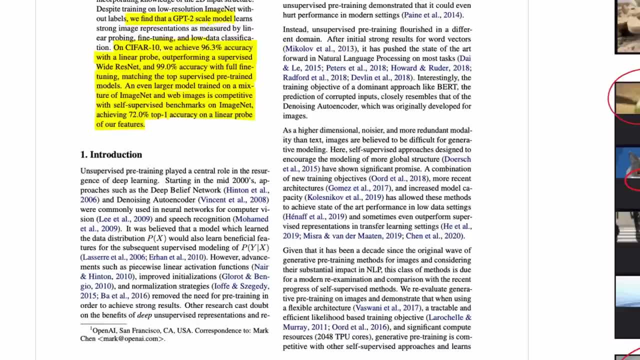 transfer, learn it to classification tasks, And the point of the paper is to say that, like in text data, in text data we have made pretty good, pretty good experiences with doing this, with pre training, a generative model and then fine tuning on a classification task, While so far, 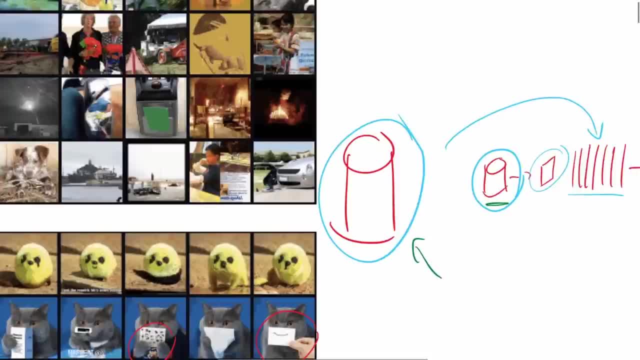 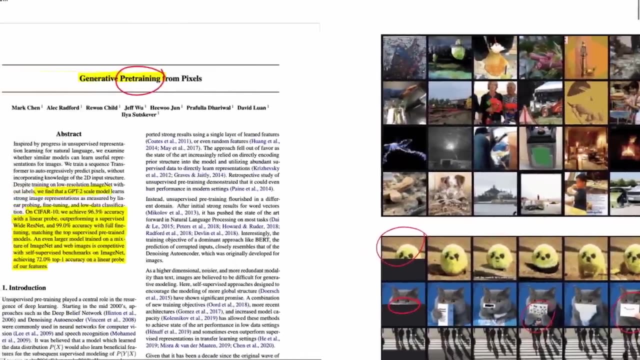 in images. all we've ever done is we've pre trained. These pre training tasks usually is a classification task or like a self supervised task with a contrastive loss or something like this. What they're doing new is the generative modeling in the as a pre training. And again, 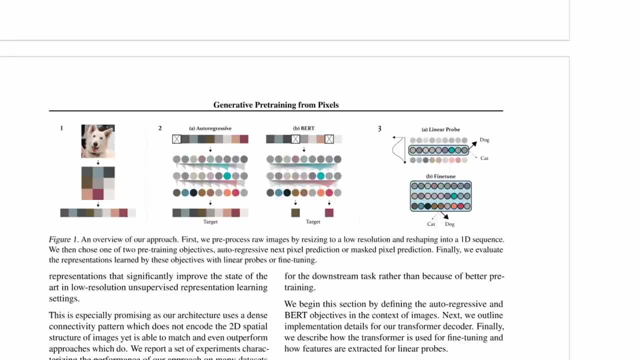 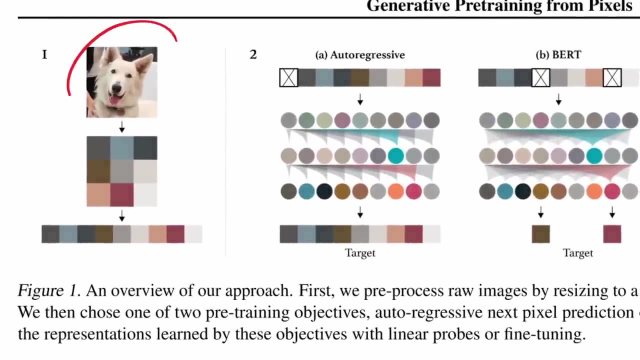 this isn't like entirely new, but they show that if you throw a lot of computers at it and lots of data and a big model, then that can work equally well to the self supervised tasks. So their model, as I said, is pretty, pretty simple: They take an image and they unroll the image. Now 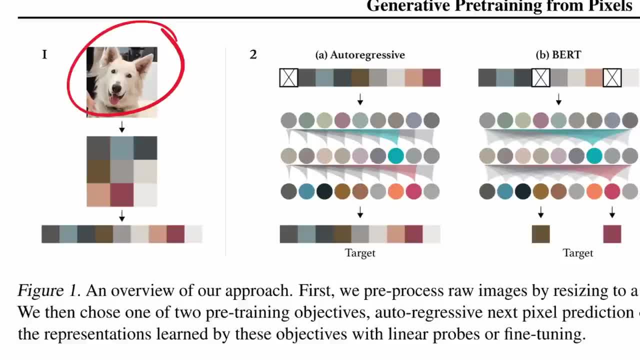 a fully unrolled image on, let's say, ImageNet has 224 squared pixels and that times three. right, because you have three color channels. That's too large even for an open AI supercomputer. So what they do is first they downscale the image. So they downscale. it's not as drastic as here. 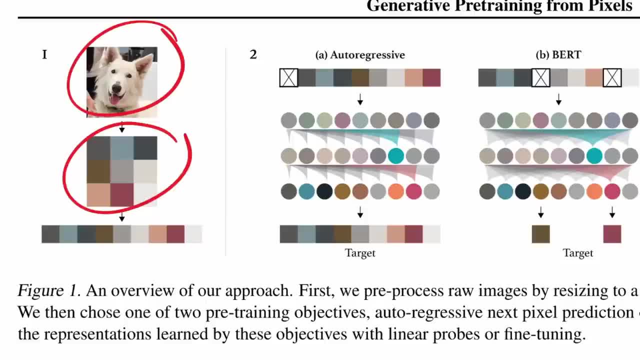 where you just get a three by three image, but they do downscale it to like a 32 by 32, or a 64 by 64. Then they unroll it, which simply means they go through the image like this and make a: 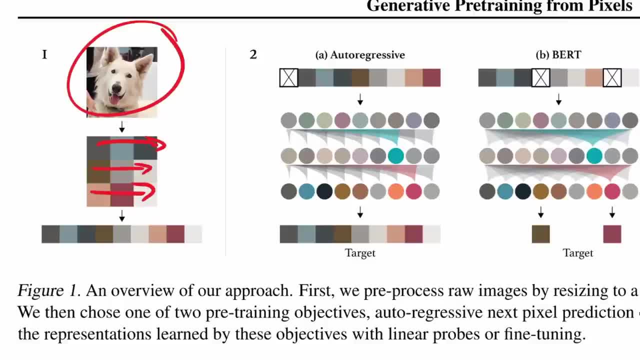 sequence out of it, because their models are naturally made for text sequences. They simply put the image into a text sequence. They further simplify this by reducing the three color channels to a single one, So they have their own color representation And basically, yeah, they reduce the three color. 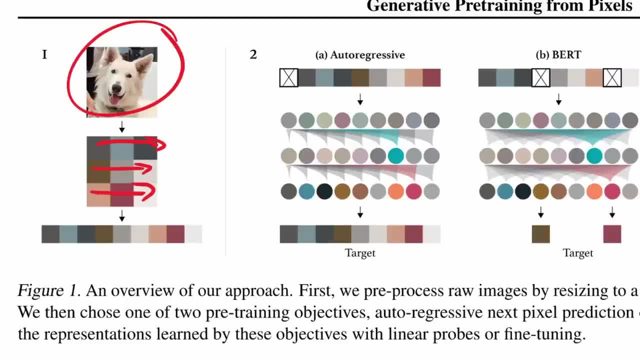 channels, to one channel that simply indexes the color in their color representation And they say: it's still pretty good, It's pretty faithful. So ultimately they end up with like a 32 squared length representation of their image. And then they do one of two things. 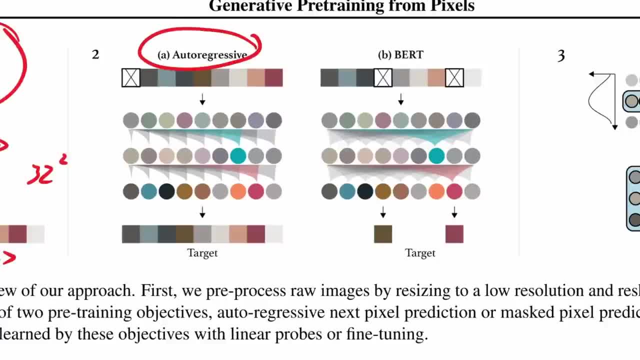 They either do one of two things. They either do one of two things And then they do one of two things In this case is the janitorbird. It does nato unexpected aging, because you can see here yourT Photo view when you zoom out, which is excited if you 무슨 style old. 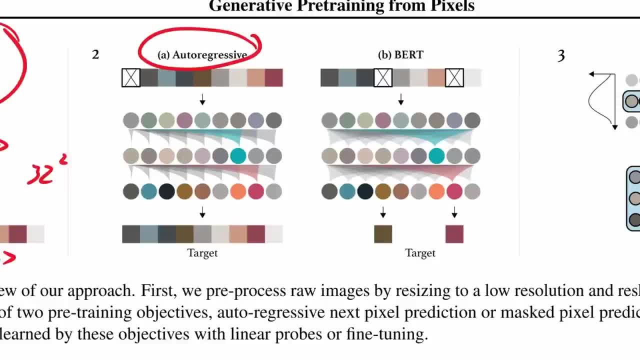 especially in this picture. it's the same cliche, obviously, But you can do auto regressive generative training. You need a, And then the idea here is that you always want to predict the next pixel of a sequence So you can see right here: that's the sequence that you sorry. 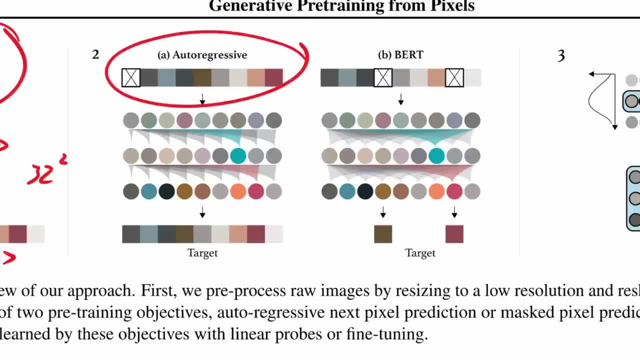 that's the sequence that you input And you always want to predict what is the next pixel And in this case, you've seen, you see that we've already predicted everything for every swell. where misguided, the Xiaiv value will be open for every group and developed. a result was 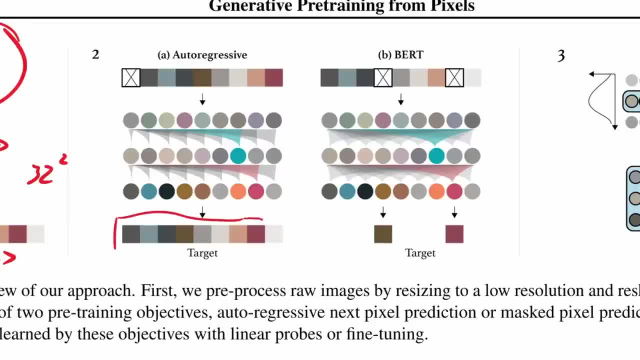 almost why you see the other style, and then you can create a pressure layeriva for each. everything here we've already predicted everything up to this red pixel, So you want to know what's this next pixel? this thing right here, What's this going to be? And the diagram here, basically, 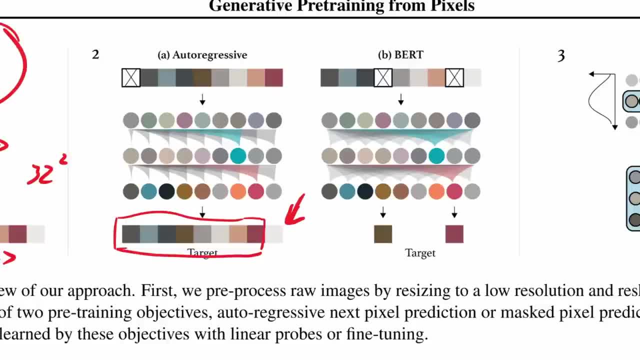 shows you how the attention flows. So every position in this transformer- and if you don't know what a transformer is, I haven't made a video about attention is all you need, where these are explained. But, briefly, every position here can sort of send information, can send information. 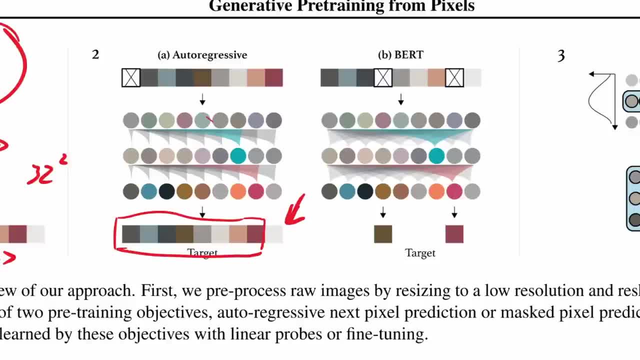 only in one direction as to. so you train all of these in parallel And when you predict this pixel right here, you only want information from whatever was before that pixel. Otherwise the model could cheat right. Otherwise the model could simply learn to copy over the value. 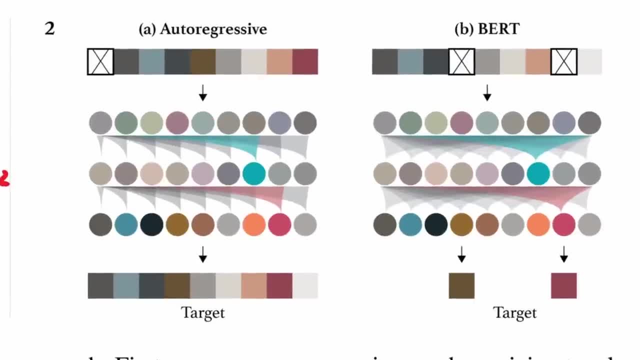 But the attention pattern here is simply to show you that this is autoregressive And it's in one direction. So you always want to predict the next pixel And then from all of this, you want to predict the next pixel, And then from all of this, you want to predict the next pixel. This is in. 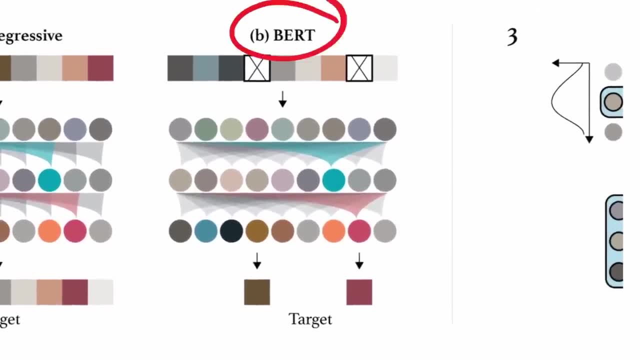 contrast to this objective here. that comes from Bert And I've also made a video on Bert. what you do in Bert is you simply take that image and you cross a block out two of the pixels or many of the pixels And you simply ask: 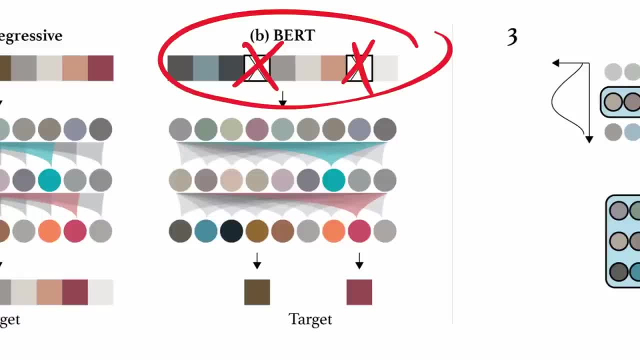 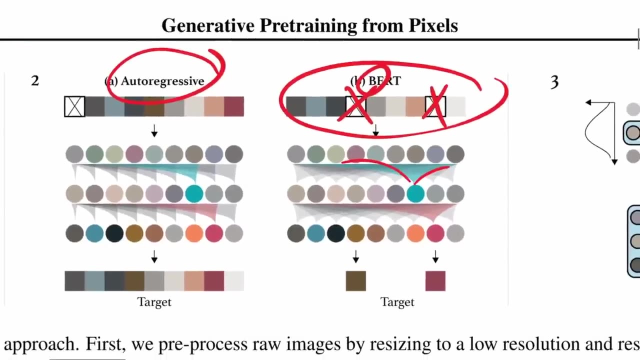 your network to reconstruct those pixels. okay, And now you can see. the attention flows in all direction, Bert. the B stands actually for bi directional, So this is the contrast to the autoregressive pre training framework. Now the these two things have been applied in text both. 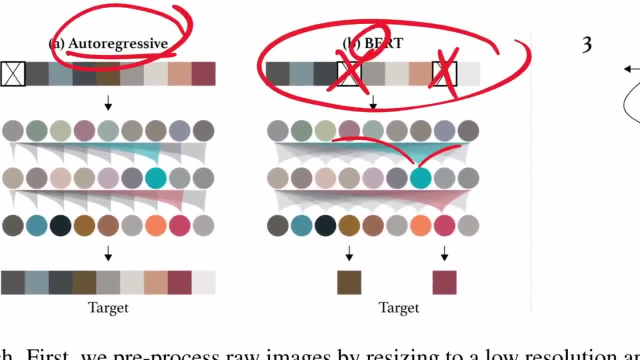 the autoregressive is, usually it's easier to actually make it produce something like we saw producing these images, Because you can always just predict the next pixel, and then the next, and then the next, and then the next, Whereas in Bert it's a bit more unclear how. 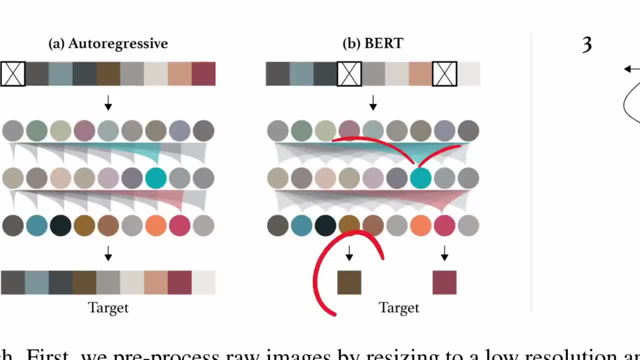 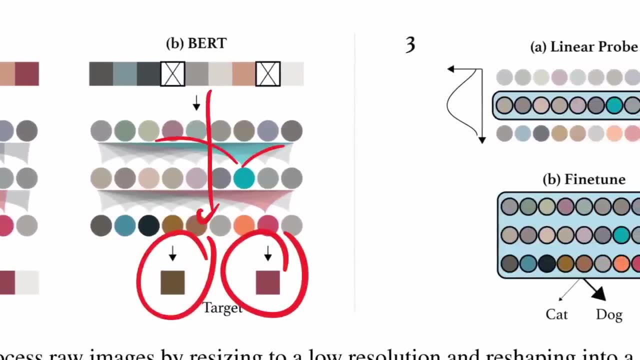 you would produce things in a consistent manner, because the predictions of these two pixels right here, they are independent. it's one forward pass and then both of these are predicted. But other papers have tried to solve this like this- Not XL net, I forget. I forget its name, it's something. 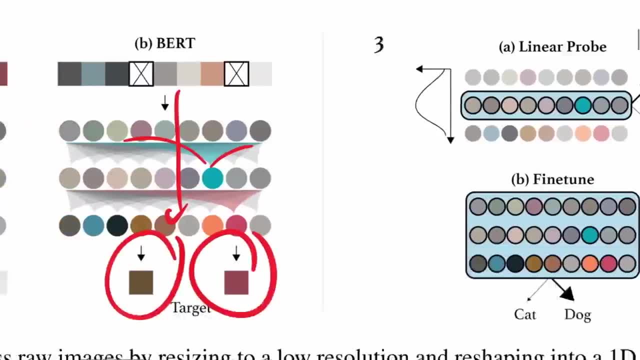 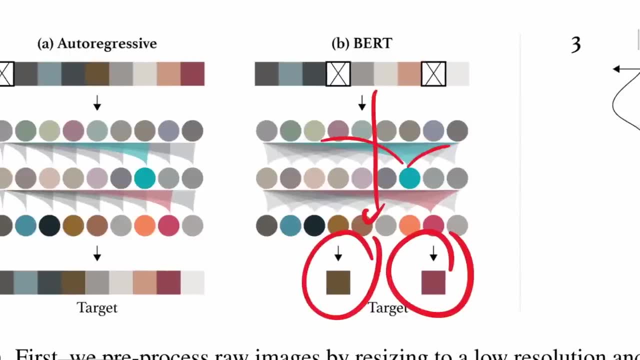 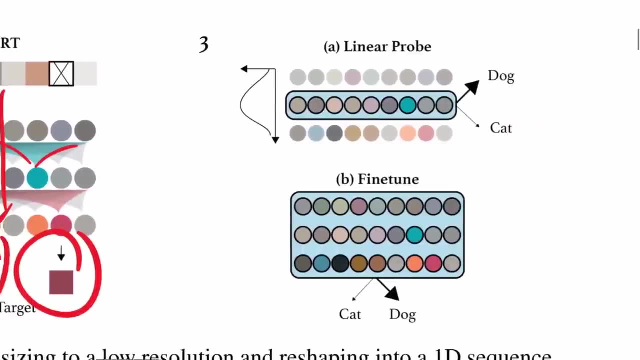 with an X And yeah, but but these are the two objectives they look at And it turns out they sort of trade off a bit. they work equally well or a bit better and a bit worse depending on the task. So once 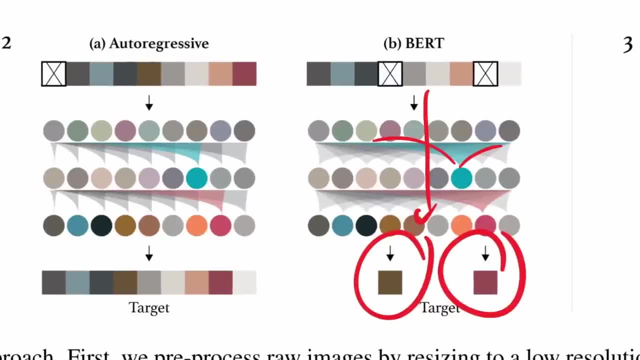 they have done this, so they simply feed images, and you will notice that you don't need any labels for this. So what you'll do is simply input an image and then simply take away half of it, like this, and then predict. 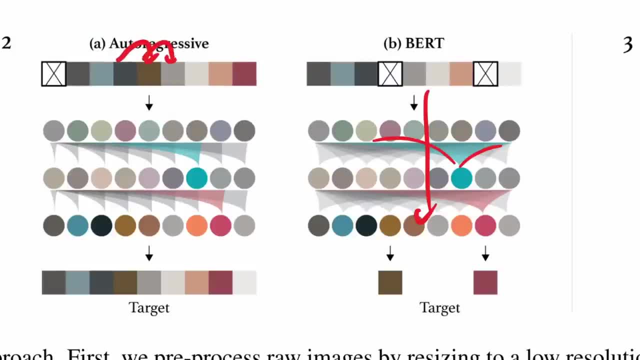 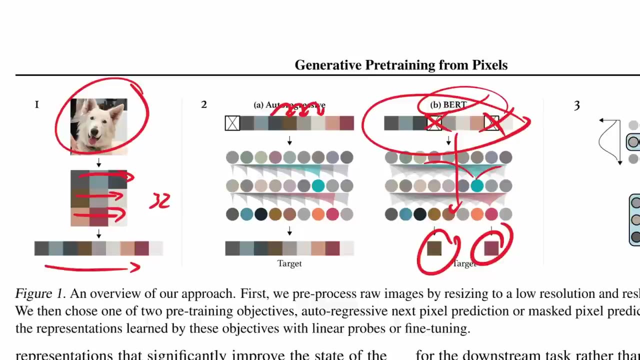 that pixel, and then you want to predict that pixel, and then you want to predict that pixel. right, That's all like you do with text, And in Bert you simply input an image, cross out pixels and then predict them, So you don't need labels for this, And that's why you can do it with this. 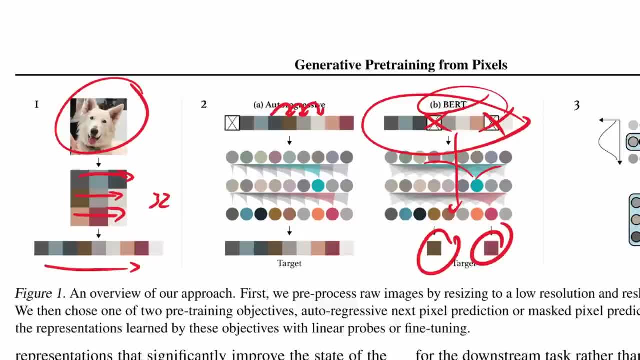 big data set And you can do it in an unsupervised fashion. So you can just crawl the internet for for images and just feed this in into there And it will sort of learn to produce these images. Now the question is, if you produce, if you learn to produce these images, does that? 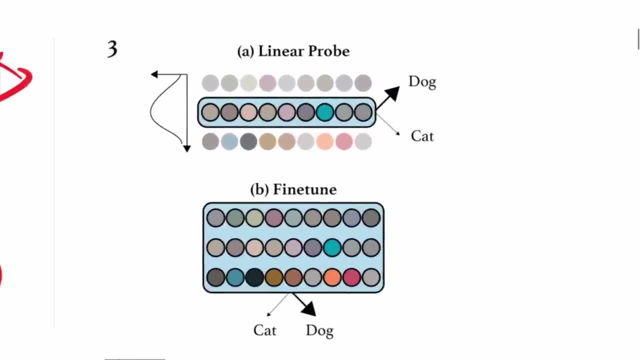 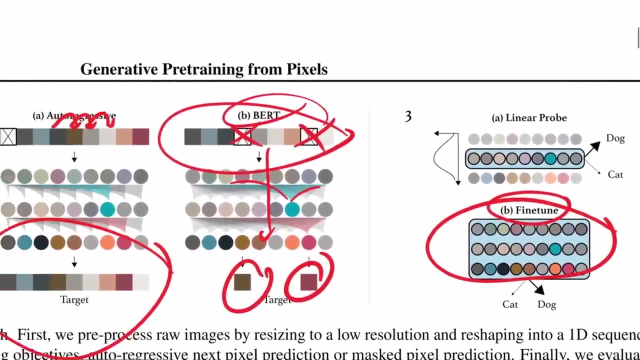 help you for classification. And there they have two methods of of assessing this. The bottom one here is the fine tuning method, where you simply: so this is supposed to be the representation you learn in the different layers of the network. So this is supposed to be this thing right here, What? 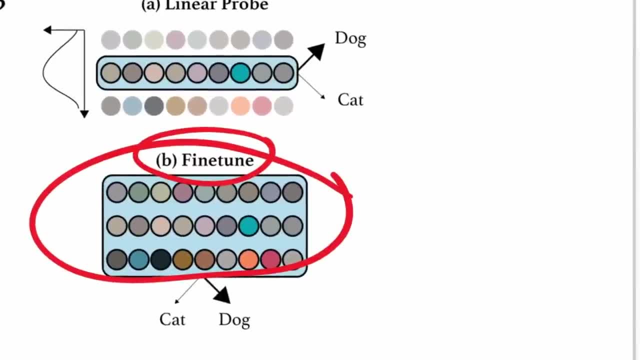 you'll do is you'll simply fine tune. that means you, on top of this representation, you add a classification head that has two outputs- cat or dog- And you train this entire network on your small data set that we discussed before. So you train the entire network, all of the parameters. this is called. 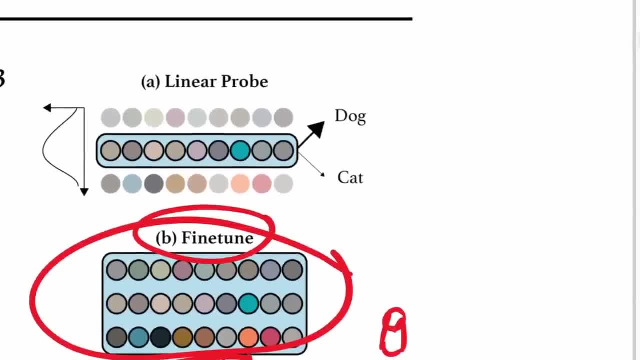 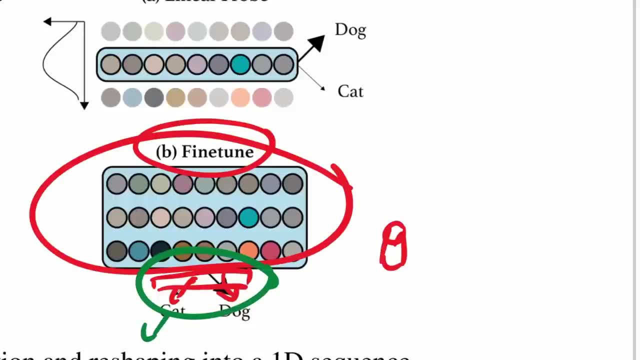 fine tuning. In contrast to that, what you can do is you can simply- and this is the easy way- you can simply add this classification head with two outputs and then only train this classification head, And that is won't perform as well, But it gives you sort of a better idea. 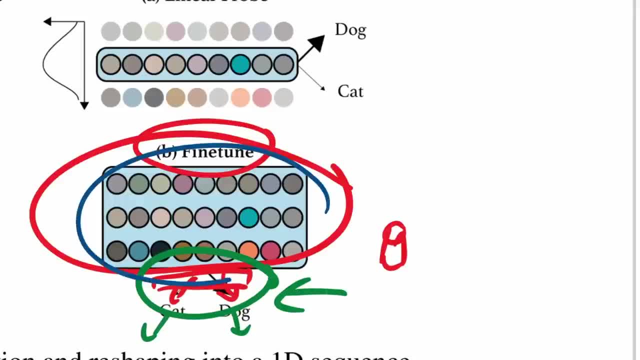 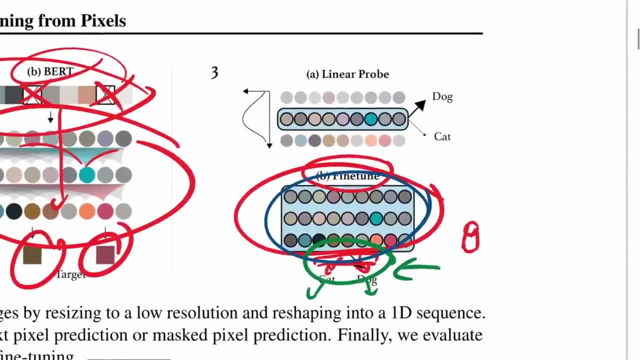 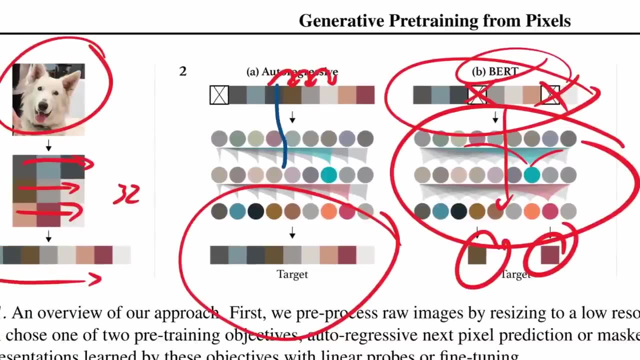 of how good is the representation that this network right here learned. And on top of that, so if you spin this idea further, you can actually go and do this at any intermediate layer right here, So you can forward, propagate until layer two right. 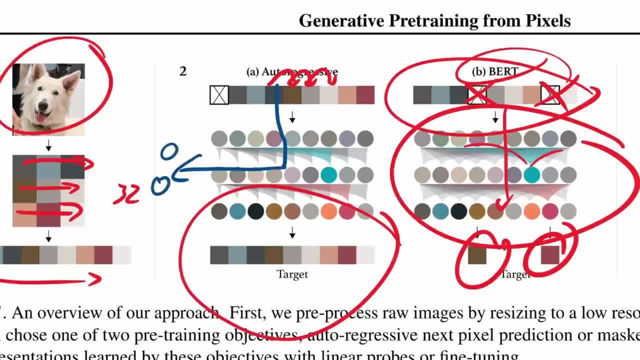 And then here you add your classification head into the two, into the two classes, and you only train the classification head. That being said, you can also do this with fine tuning, But in this case this is called a linear probe And it is often used to assess how good the a representation. 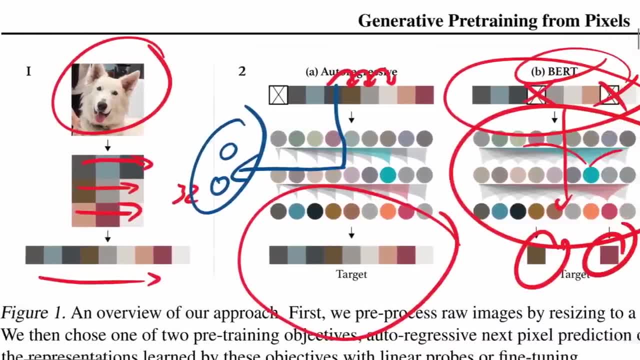 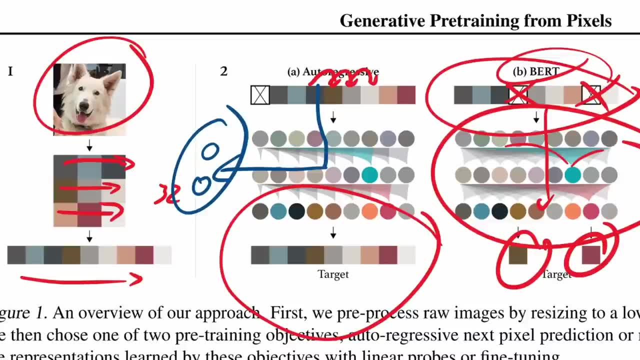 in intermediate layers is, whereas what it actually does is assessing how linearly classifiable a representation is, which is a linear representation, And that's what we're going to do here. So this isn't the same as how useful or how informative, but it is one way to to assess. 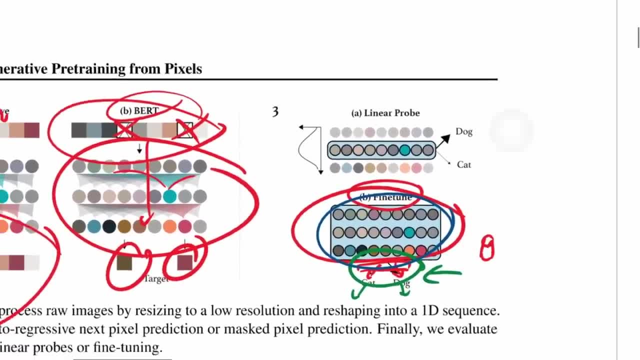 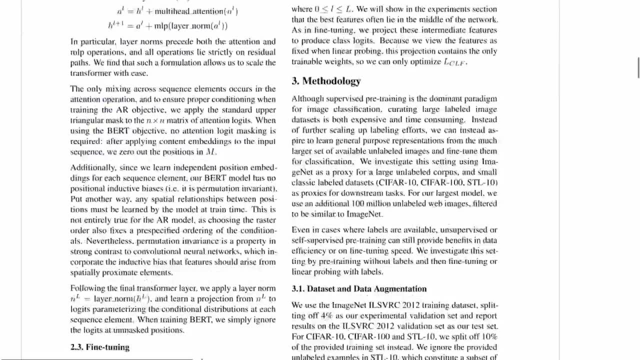 these things. Okay, So these are the two things they assess. Alright, so for as for data sets for C for 10, they use, like C for 10 and C for 100 as data sets, and the STL 10.. And there you have to. 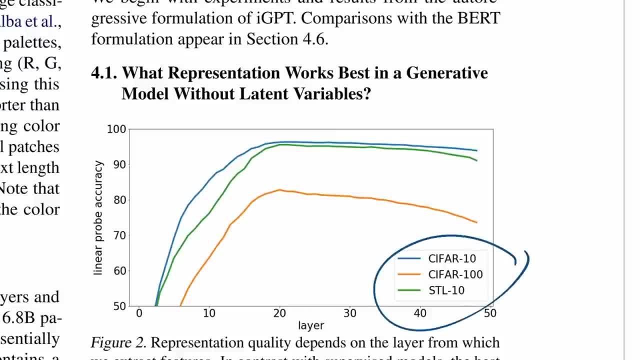 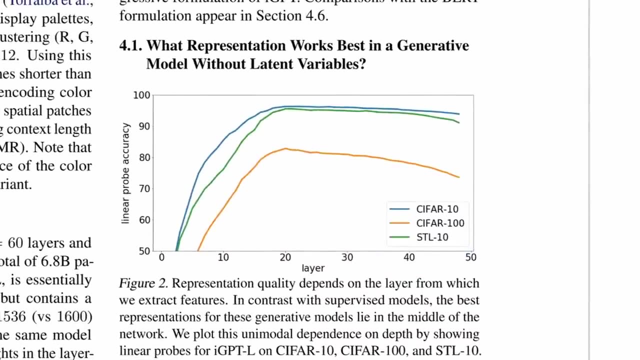 keep in mind, the pre training is done on image net for those, so that you pre train on image net without the labels And then you transfer, learn or fine tune or or linear probe on these small data sets, Whereas later we're going to look at image net. in there, the pre training, as I understand it, is done on 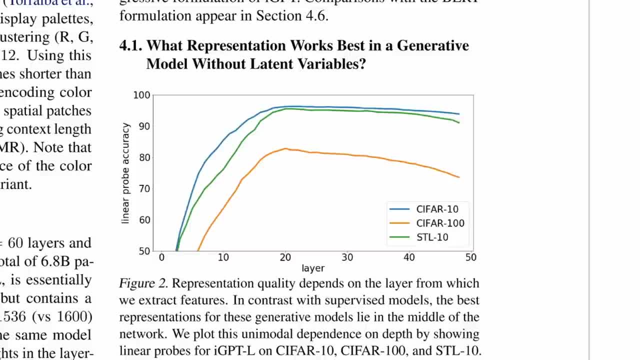 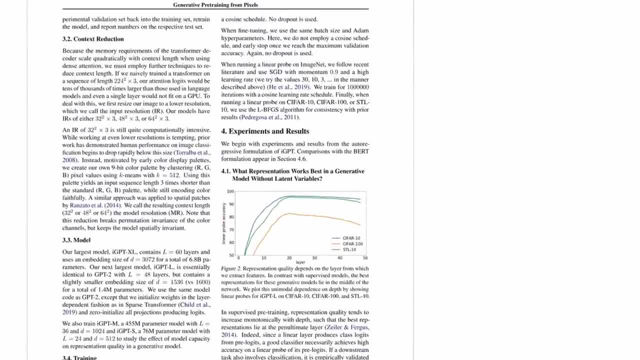 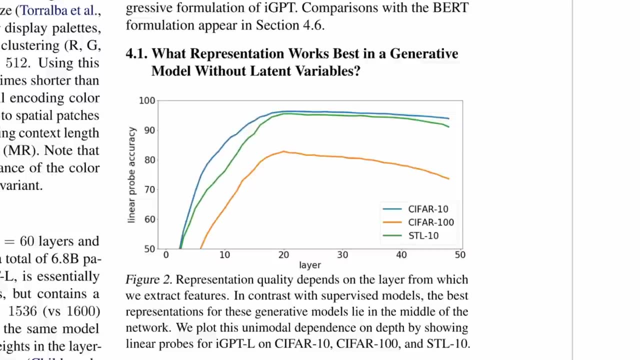 image net itself, but also a wider collection of a hundred million or so images from the web, from the internet. Okay, So, as you can see right here, this is what happens if you do this linear probing And you can see it works pretty well. So you get: 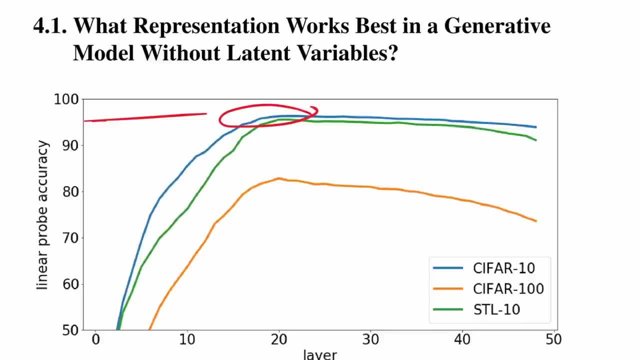 like a 95- 96% accuracy with linear probes. This is very powerful. So it's not easy to get 96% on C for 10.. I mean, current state of the art is like 99%, But still 96% is pretty good And this is the so. the state of the art is like 99%, But still 96% is pretty good, And this is the so. the state of the art is like 99%, But still 96% is pretty good, And this is the so the. 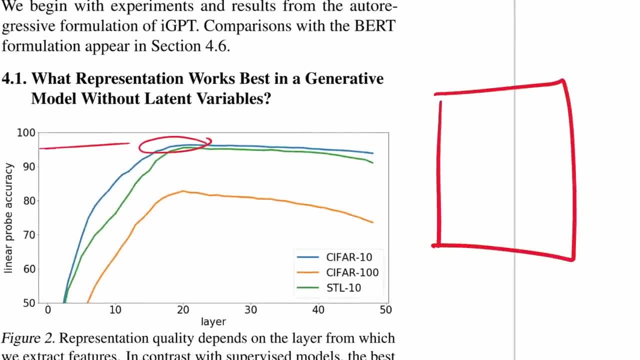 entire network. there is this big giant network that you input your image into, And then there is this one linear layer that does the classification. And all of this right here has not been trained with classification in mind. it simply has been trained to reproduce images. It hasn't even been 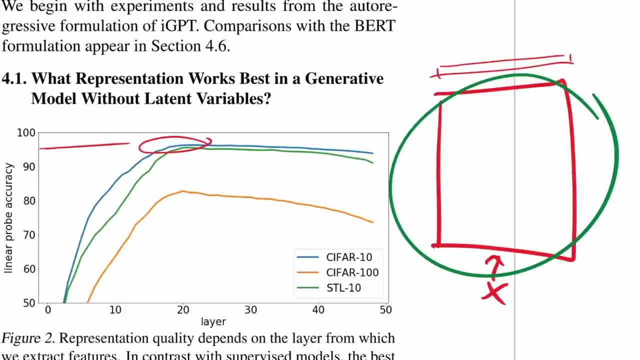 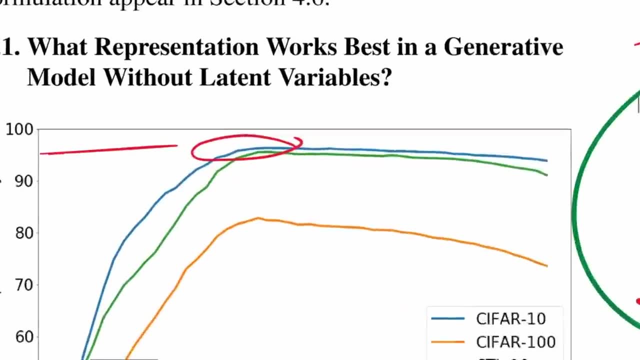 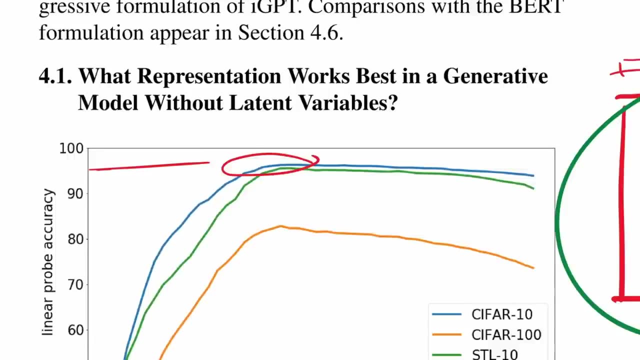 trained on C for 10.. As far as I understand, it's been trained on image net. So the the this is to stress how cool or how significant this result is, basically that just a linear probe on top of that will give you such a good accuracy. And the second thing that is obvious right here is this bottom: 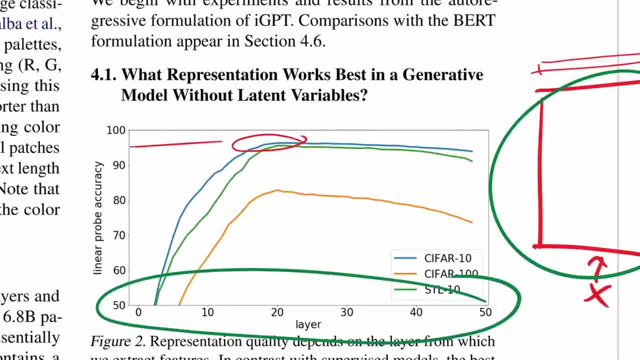 axis is the layer, So this is the layer where they attach the linear probe. And usually if you pre train a network with a classification task in mind, so you pre train it with the labels, or maybe even without the labels in a self supervised way or something like this, usually the last 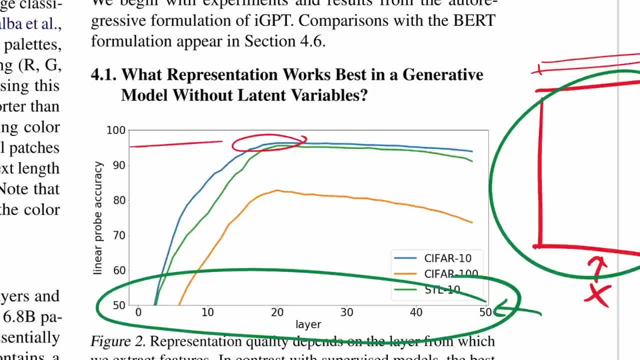 layer has the best representation for classification. But here the special thing is that the intermediate layers in the middle have the best representation. you can see that the representation quality in terms of linear probing falls off as they sort of it, falls off as they go. 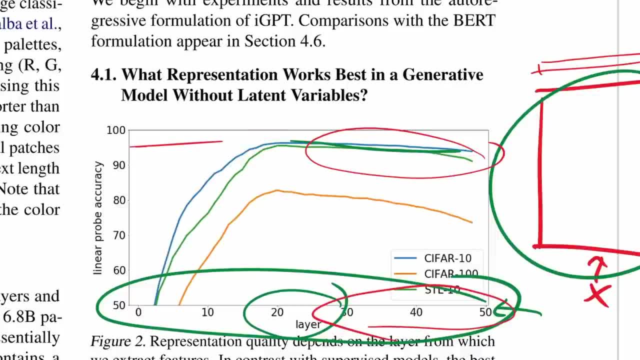 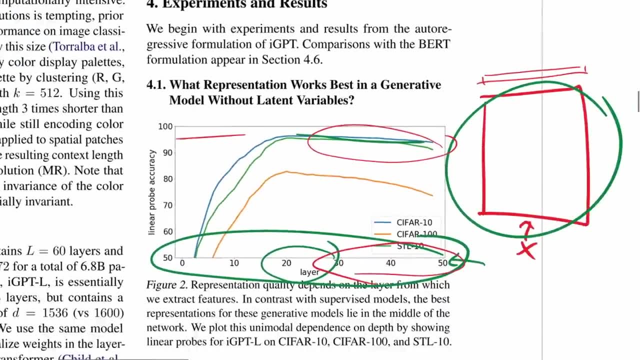 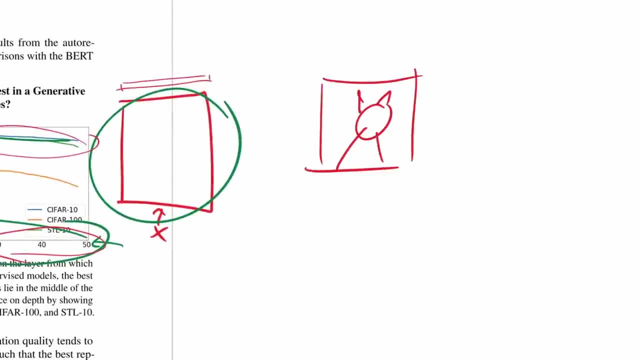 into higher layers, And this is consistent across the data sets, as you can see, and the. the idea here is, or the way they interpret it, is that if you have an image right here and the, you've blocked part of it, so you've 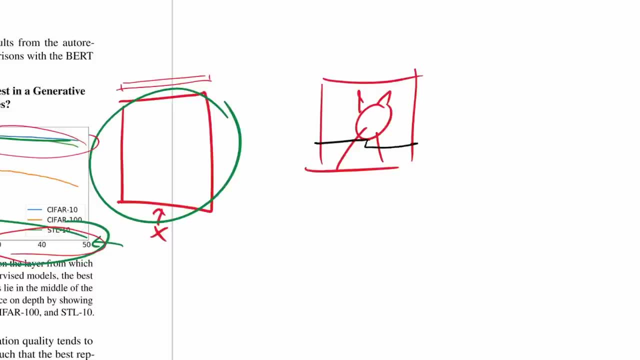 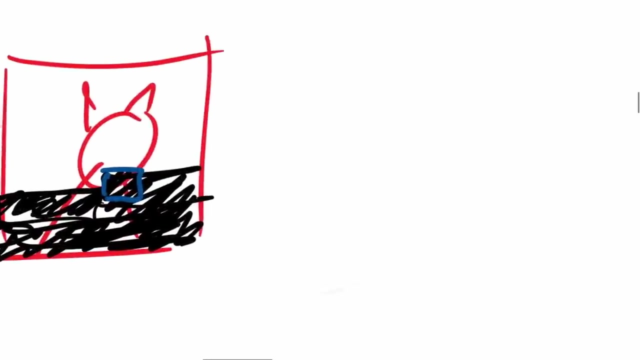 blocked this and this wrong way around this. So, no, you've generated everything and now your task is to predict the next pixel. right. So you're you train to predict this next pixel, right here, And the idea is that, as you put the image through the network, what it will do is 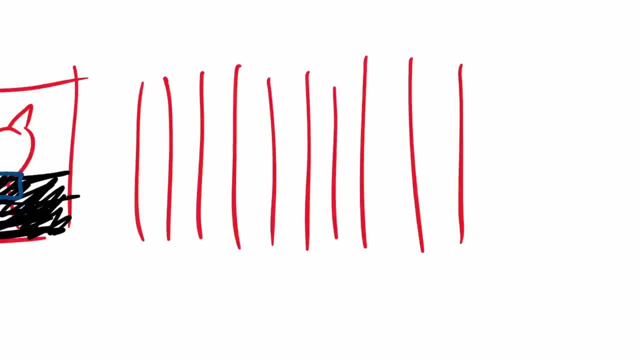 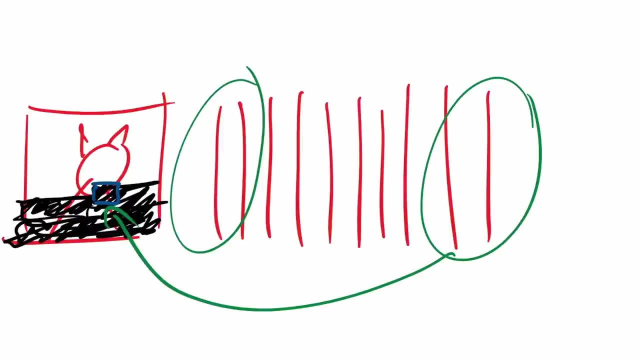 sort of, since the first layers they're going to be- they're going to be similar to a CNN, they're going to be doing some low level feature transformation thing, right, But also the last layers they're going to really care about what's the exact pixel that goes here. 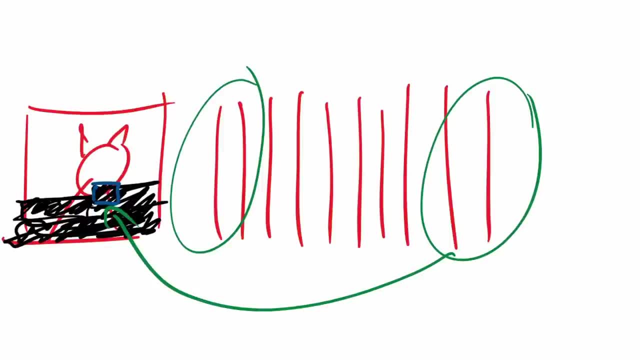 right, Since it's their job to do, that, they're going to care. what color does it need to have, you know what exact luminosity, and so on? how does it fit in with the previous pixels and so on? where as so? that's, that's. 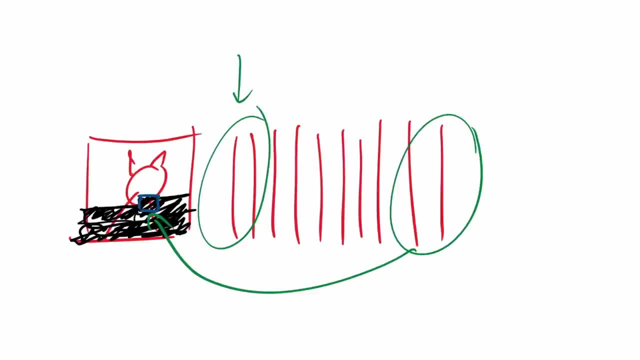 also good, but it's not just low level information and consistency with other pixels or something like this. At some point, if you want to generate consistent images- and we saw that this model can generate consistent images- at some point there needs to be some kind of a notion of the global information in the 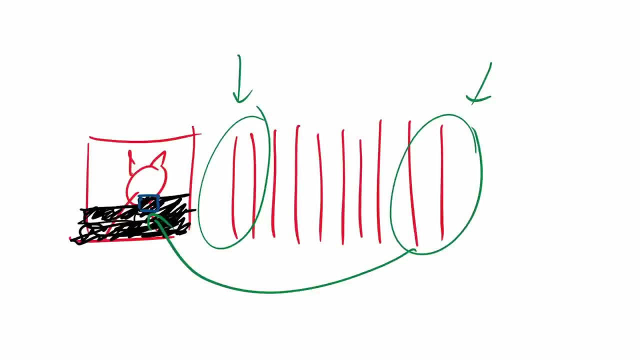 picture right Such because the images are consistent throughout. So there needs to be some, some notion of what is in that image as a whole, And that's the exact information that we need for classification, And the only way that could actually be is here in the middle, since, you know, that's the place. So the hypothesis is that 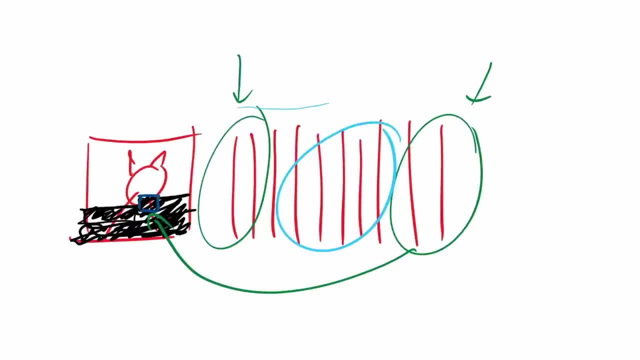 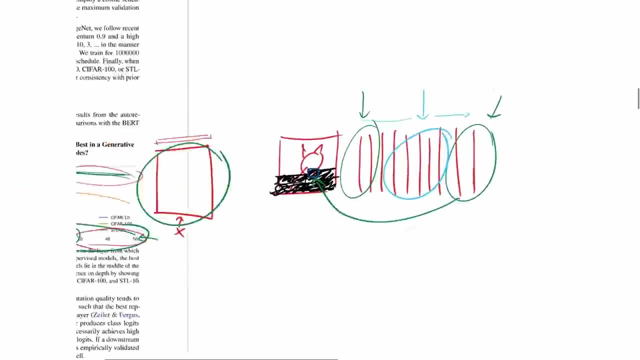 the. these models somehow learn a higher level representation of global information somewhere in the middle before they then specify that information again down to predict the actual pixel, And that's why the best representations for classification are in the middle. So this is one of the. this is actually. 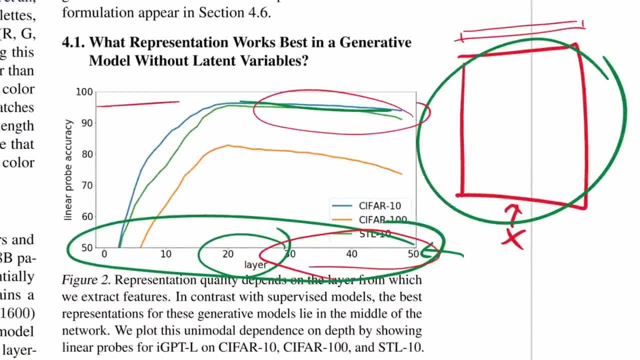 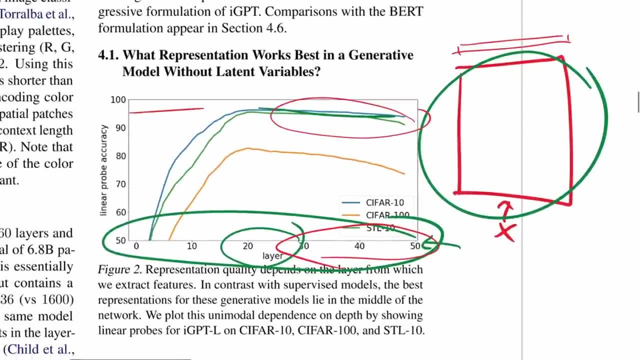 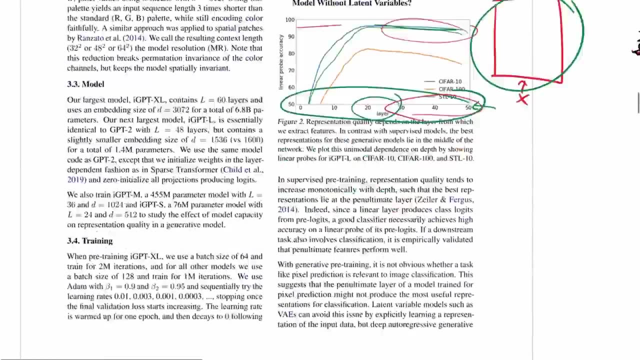 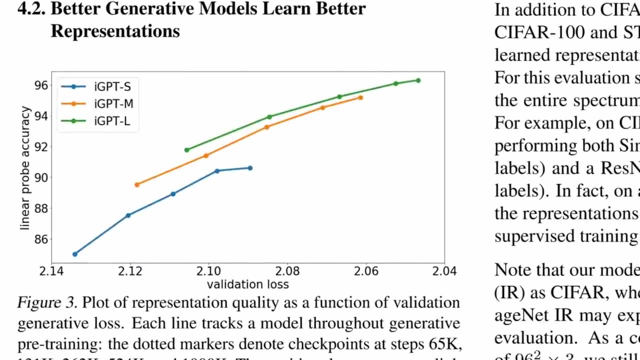 the interesting finding, or one of the interesting findings of this paper. I mean it's cool that they can reach a good accuracy, But to recognize that maybe in these, these generative models, they have some intermediate stage where they represent the global information and that will actually make the best representation. Okay, the second cool thing right here is that you can see they. 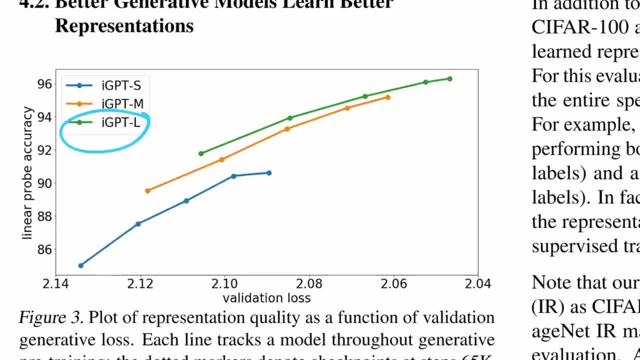 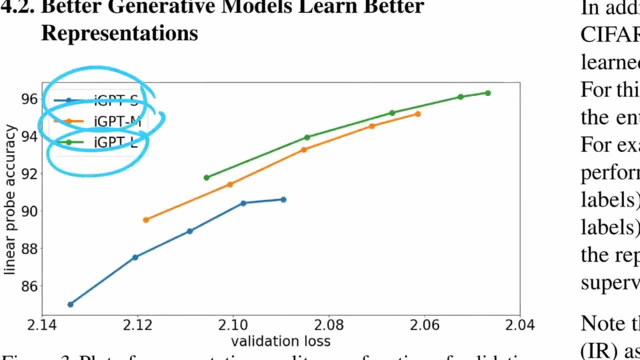 have different sizes of models. So the IGPT-L, I believe, is something like 60 layers, then this is like 48 layers and this is 32 layers- we don't really. So these are on the all of, on the scale of GPT-2, either a little bigger or a little smaller. it's not like a GPT-3 scale where you need a ginormous. 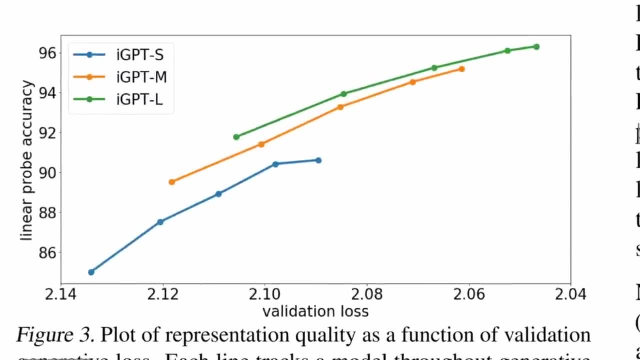 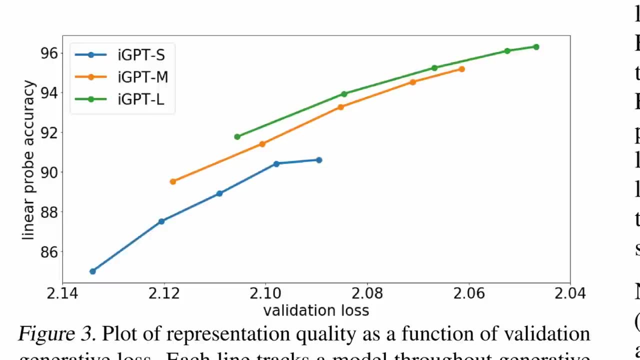 supercomputer, though they do do a lot of computation. But this still sort of fits within hardware, hardware of a standard size and not like exascale. What's interesting right here is that you can see the larger models. they reach a lower. 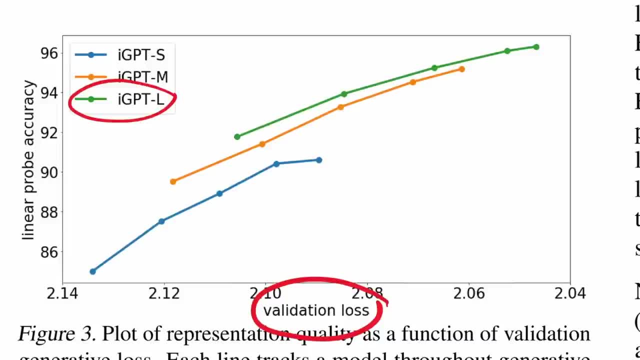 validation loss. So here is the validation loss larger model, if you train them on. So these checkpoints here are always: after the same amount of steps, the larger models do reach a lower validation loss, right here as you can see. So this is the large, this is the medium. 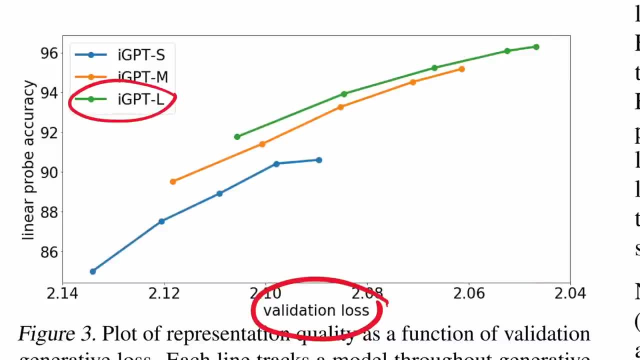 this is the small And also you can see that on this axis- the linear probe accuracy. So this is, whenever you you go and you find the best intermediate layer for linear probing, you probe it and you record the accuracy So you can see a general trend as your validation loss goes down. the linear probe accuracy. 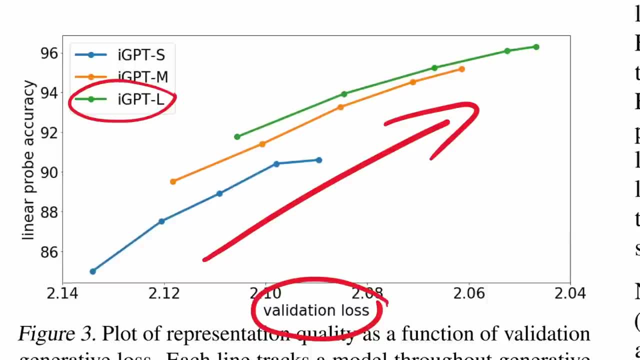 goes up. So there is a connection, like it is in text models. In text models there's a connection of the perplexity of your language model and the quality, that of the representation you get for downstream tasks In this model. it seems to be the exact same thing. there is a connection between reaching lower 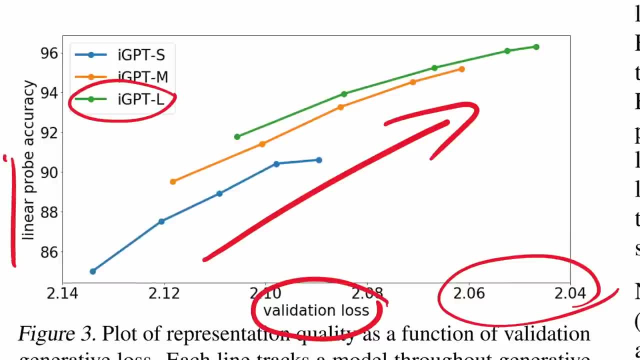 validation loss and reaching a higher performance on classification. So that's one interesting thing: the general trend to up to the upper right corner. The other interesting and even arguably even more interesting thing is that if you look at the other interesting and even arguably even more interesting thing is that if you look at the 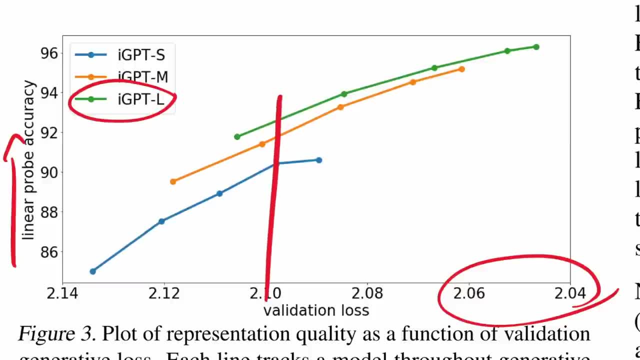 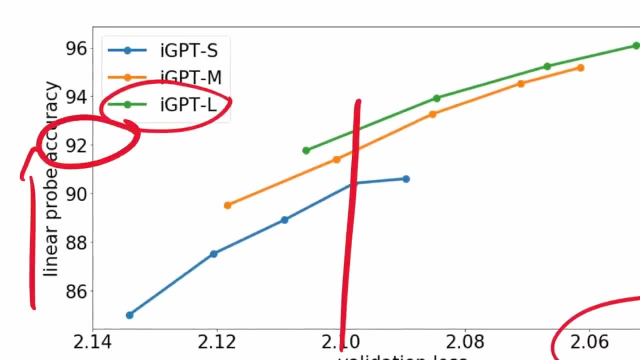 same validation loss. so at this point all of these models have the same validation loss, yet still the bigger model is better. right, you can see right here the bigger model outperforms the smaller model, even though they have the same validation. 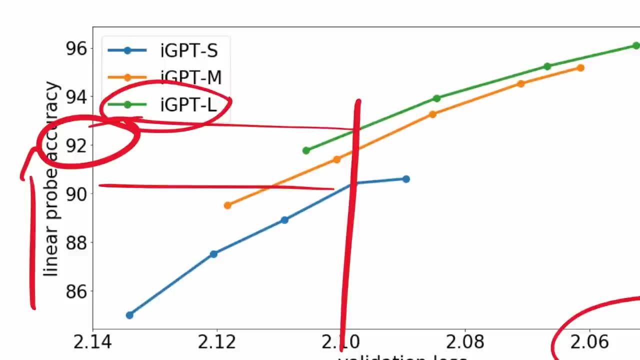 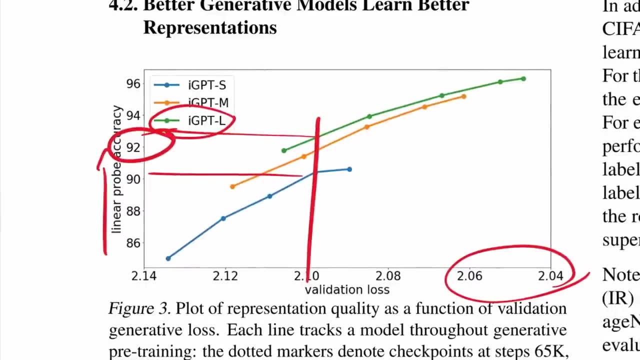 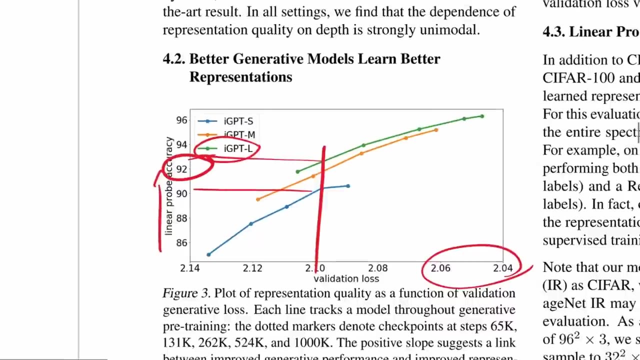 loss on the Image Modeling task, And this is also something that OpenAI, in their in their text papers, has stressed, that the larger models, they seem to be somehow more capable of forming good representations, even, you know, even if they have the same loss. 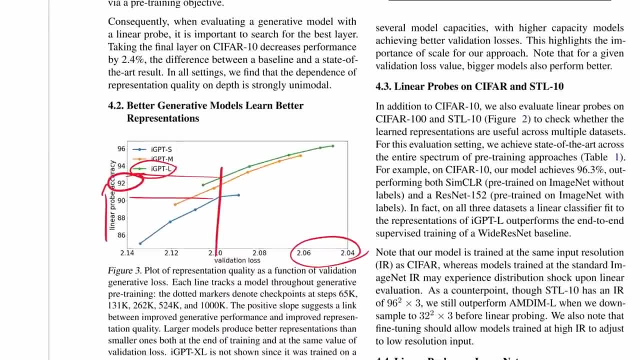 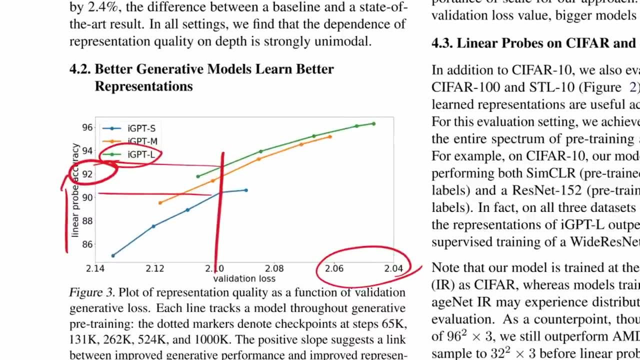 So again this: this could just be sort of a training data, better training data remembering thing. And when I said that in GPT-3, I didn't actually mean explicit remembering of training data, I meant kind of a fuzzy remembering of training data. I've I formulate that in the 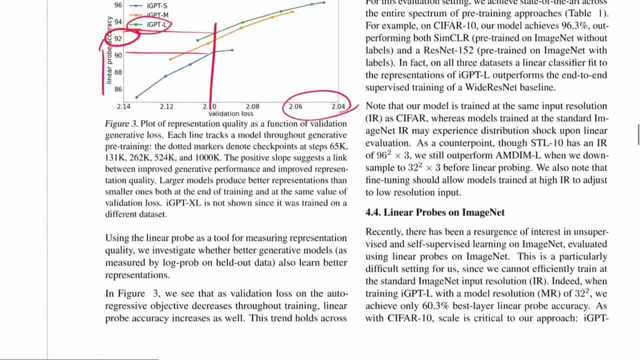 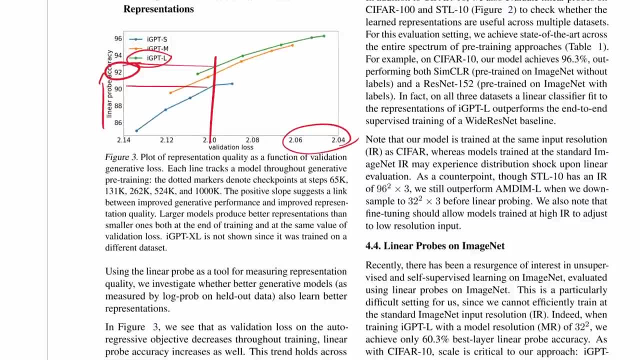 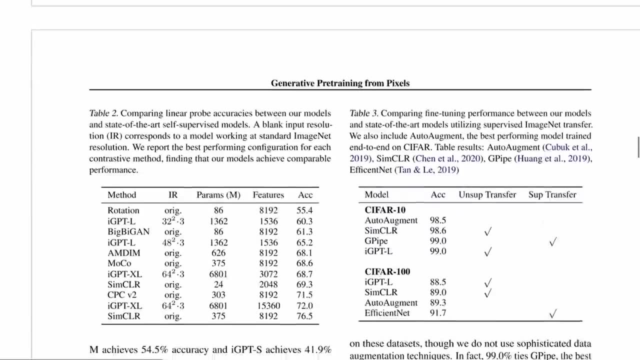 in the comments, but I I feel a lot of people have misunderstood me there Here. I think it's much harder, harder to estimate what's going on. Also, since image pixels- humans don't have a super good model on image pixels in their head as we have about text, As you can see, if you then. 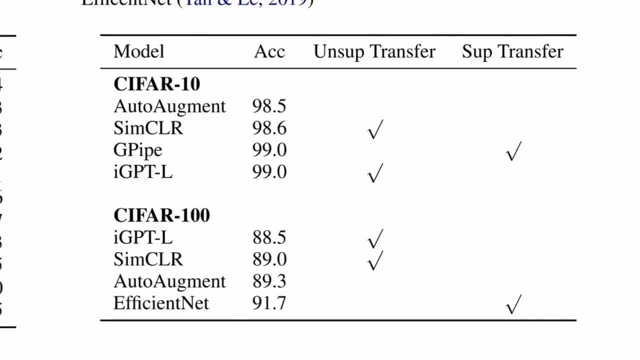 fine tune. so for now we've just do linear probing. If you fine tune these architectures, then you reach like a 99% accuracy on C for 10, which is on par with the best models that we have. So G pipe is supervised. 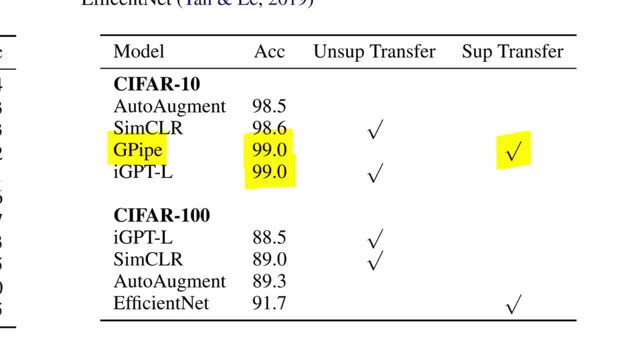 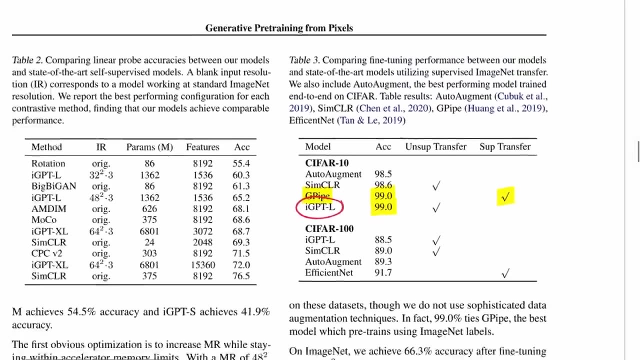 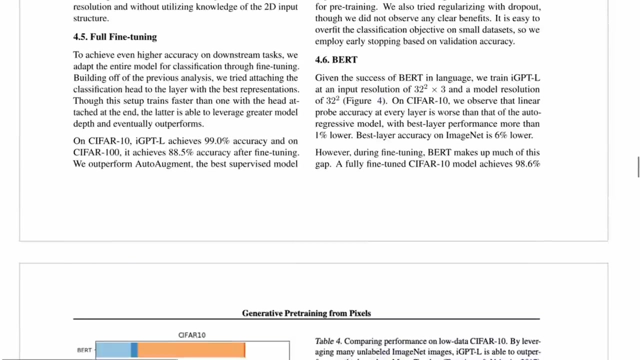 pre trained on ImageNet But also, I guess, uses a bunch of data augmentation, while these image GPT it uses minimal data augmentation. I think they simply random crop a little bit And that's about it. So they also experiment around with this BERT objective. So until now, this was all the this was. 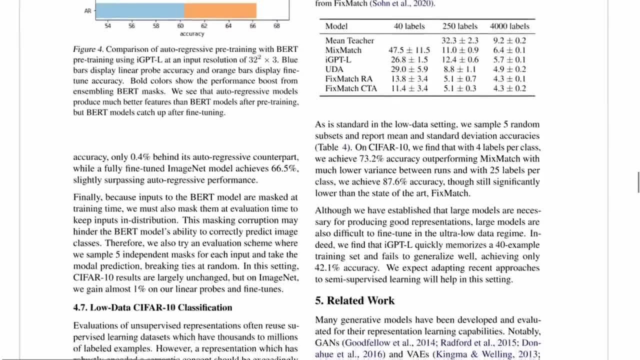 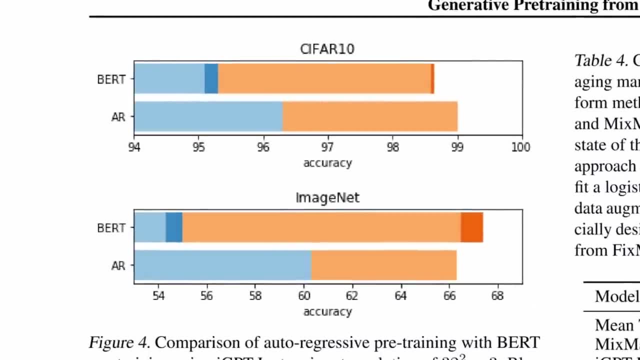 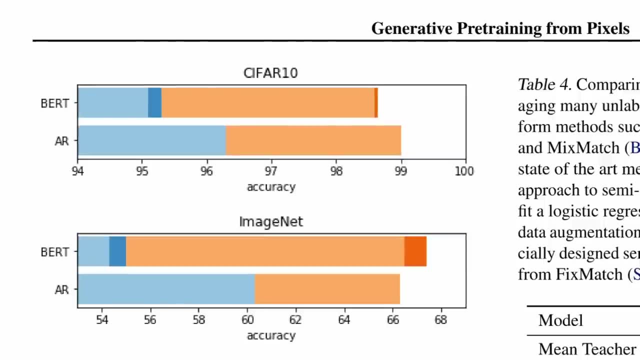 all these autoregressive objective And I feel the open AI people are a bit more of a fan of the autoregressive objective, just given what they've done so far in their papers. And you can see here comparison of the two objectives on C for 10.. And on ImageNet Again. 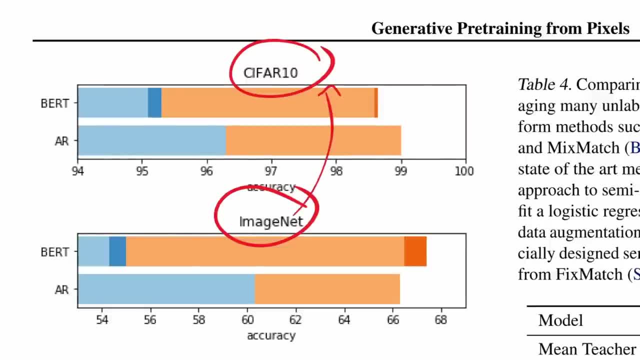 that's the only difference between the two objectives, But in any case, the image net is pre trained And the image net itself is pre trained with like a larger collection of images from the web. all the pre training is done without labels. Now, the blue is what you can reach with a linear probe And the 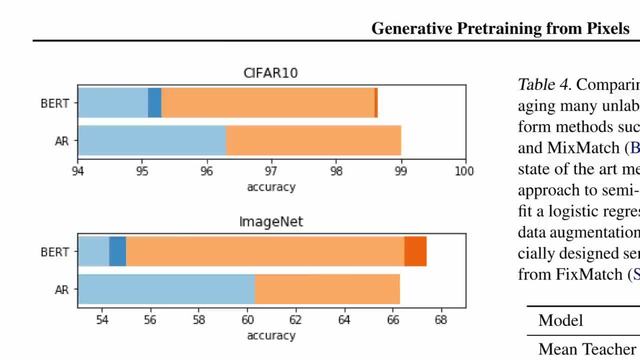 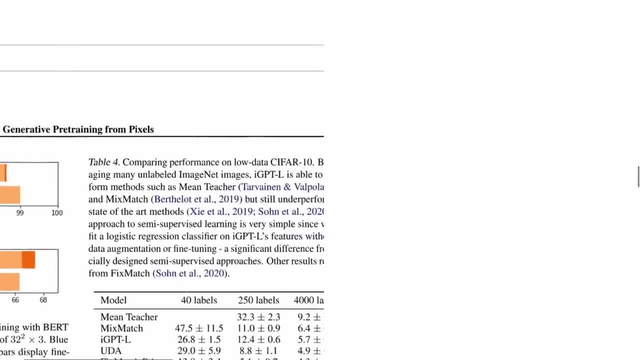 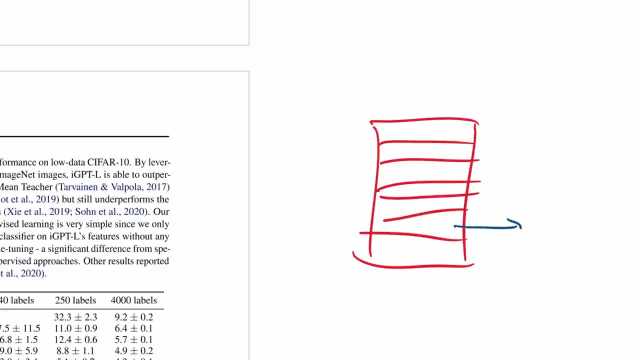 orange is then, on top of that, what you can reach by fine tuning. Okay so, no linear probe, but fine tuning, I have to say that the fine tuning is always done at the end. So, even though the linear probe, even though the linear probe can be attached anywhere in between- and it's often useful to 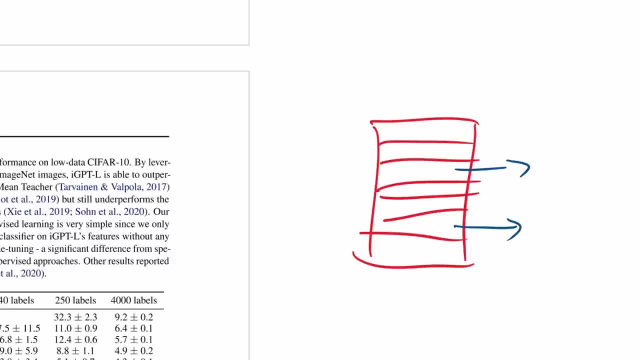 do that, as we saw, because the in-between layers are the best. they say they tried fine-tuning also in from in between, but it always worked out best whenever you fine-tune. whenever you fine-tune you take actually the last layer. so that kind of gives you an idea that the model 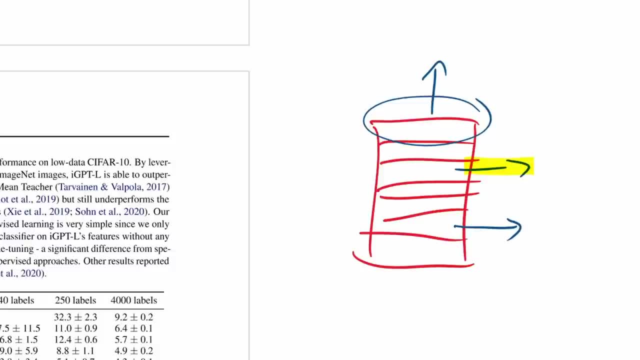 is, then it's sort of: what seems to be important is this coming up with the higher level representation, and then, once you fine-tune, you're probably able to push that representation through to the end because of your training signal. but if you hadn't done the pre-training, 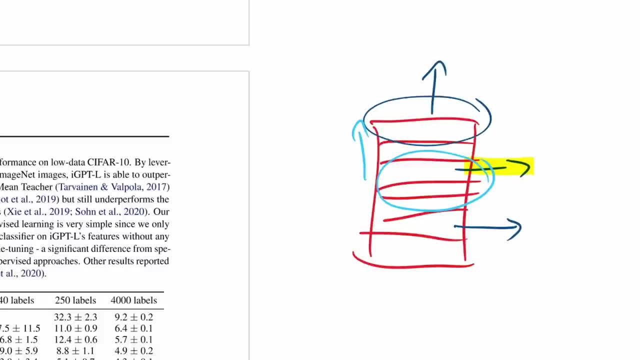 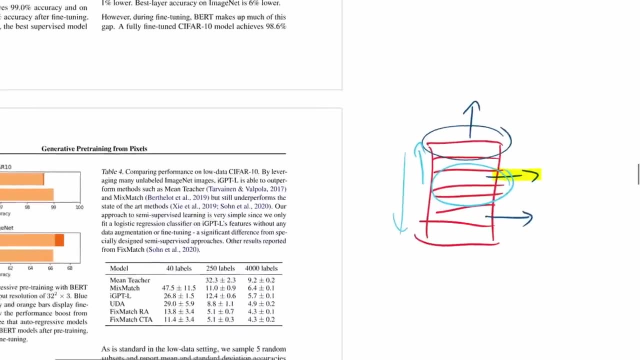 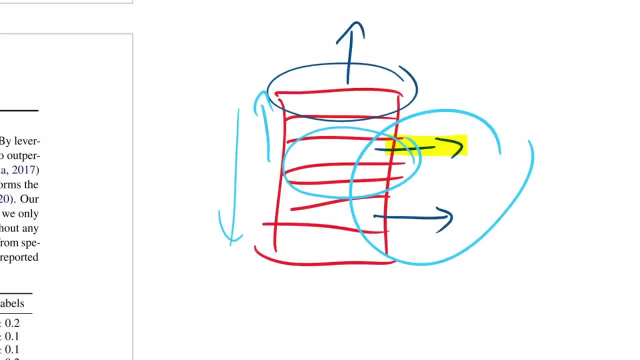 you wouldn't even have that higher level representation and then the signal I guess is not strong enough to back propagate through the whole model. It would be very interesting if they investigate, if they do this linear probe analysis again after they fine-tune the model, that, and to see if then still it is the intermediate layers. 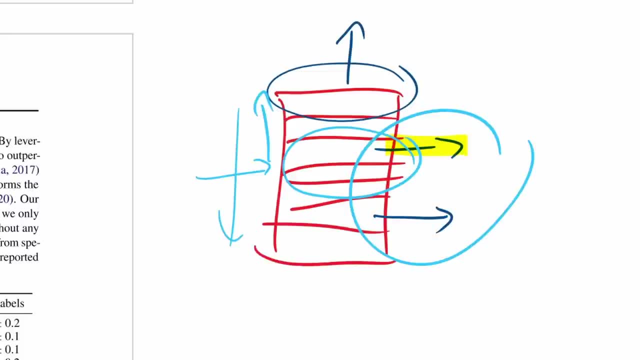 that have the best representation, or if now the best representation in a linear probe sense shifted towards the end. I'm going to guess it's shifted towards the end, but I sort of want to even see if the accuracy of the model is the same as the linear probe. 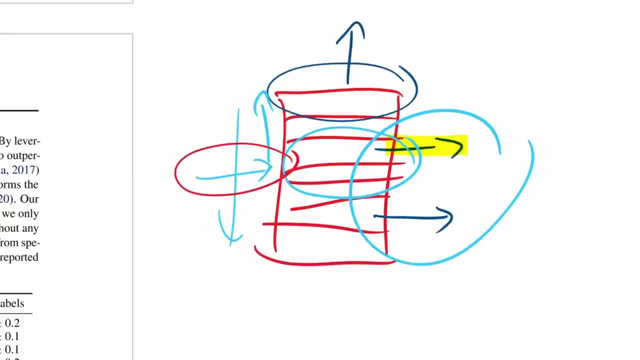 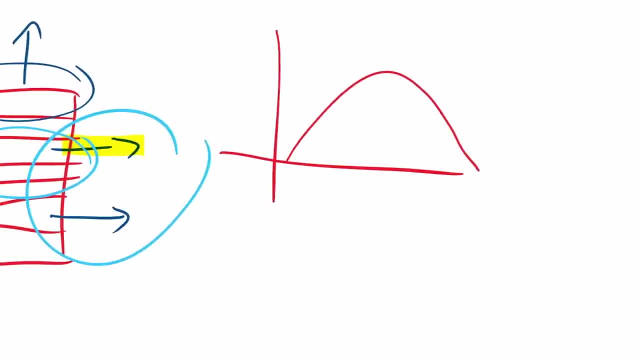 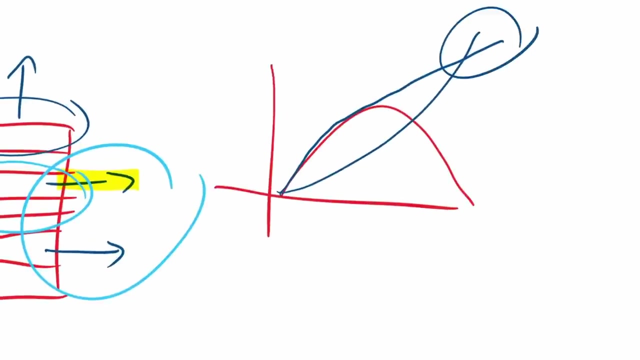 Does it keep the same? Does the curve go like this? This is the linear probe. when you simply pre-train, This is linear probe accuracy. The question would be: does it change to be like this or does it change to be like this? This is supposed to be the same at the end, So basically, 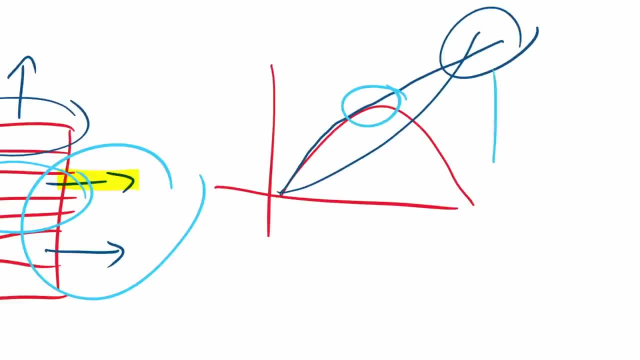 does it stay as good as it is but simply get better at the end? Or does the representation like in this curve? does the good representation now shift towards the end and leave the lower layer with even more capacity to do some low-level stuff? 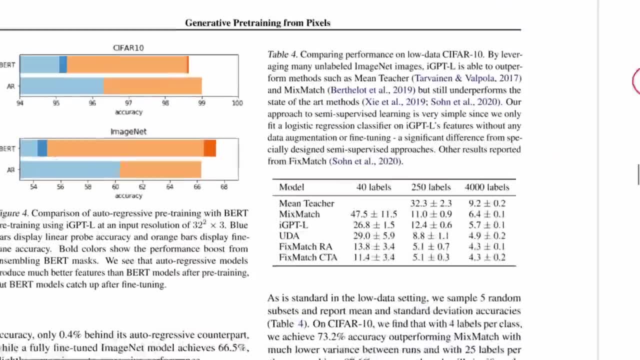 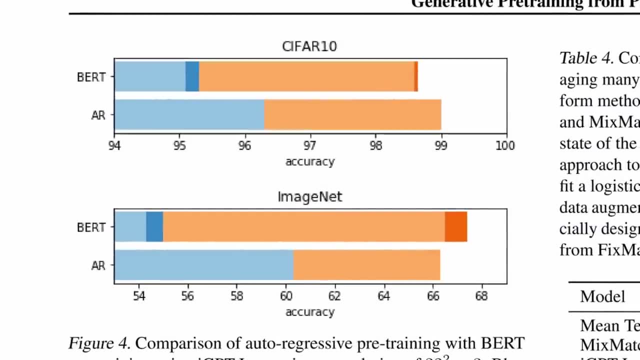 Yeah, maybe they've done this, I haven't seen it. So, and as you can see, these BERT and autoregressive objective they sort of trade off. So the BERT: it tends to do poorly in the linear probe setting, but then it catches up. 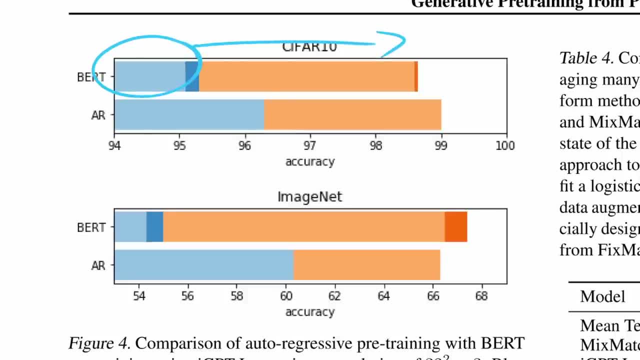 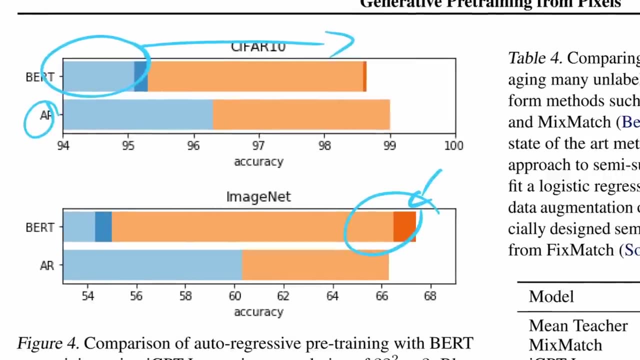 during fine-tuning In CIFAR-10, almost being at the level of the autoregressive, and in ImageNet actually outperforming it. This darker thing here. it simply means that you average across different maskings of BERT, because I guess even in classification it's not entirely. 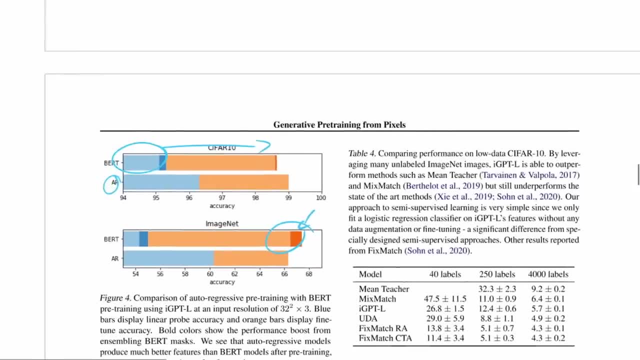 clear how to get a signal out of BERT, because they don't do this CLS vector with BERT. What they do for classification, they don't do this CLS vector with BERT, So they don't do this CLS vector with BERT. 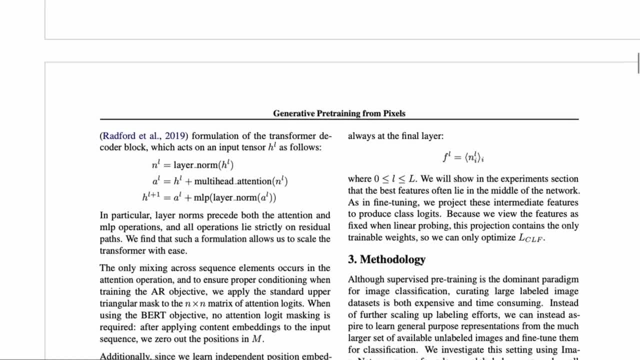 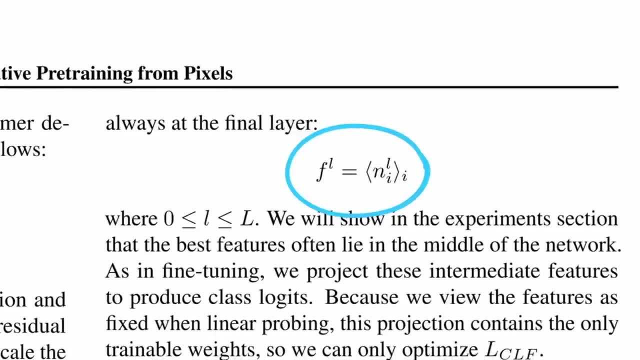 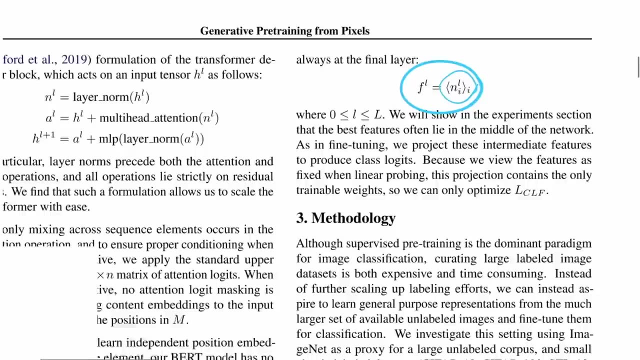 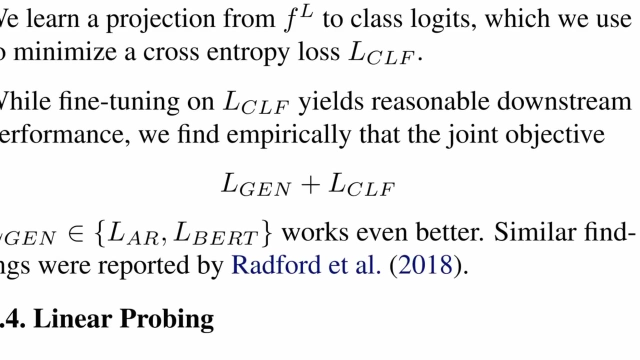 and linear probing and that's written up here. They simply take the. they do an average pooling. I think they do an average pooling of the, of all the representations of the sequence. And the last thing that I've also forgotten: There's a lot of stuff When they fine tune, while 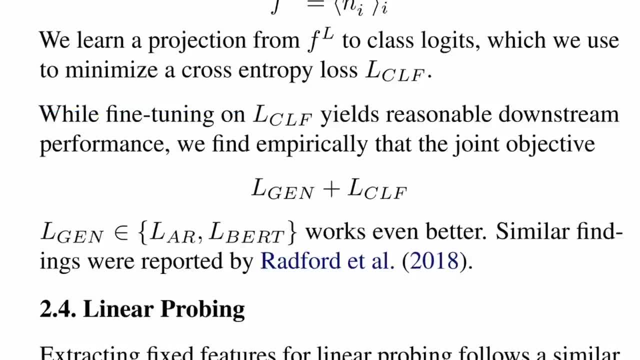 fine tuning. Come on, While fine tuning the classification loss yields reasonable downstream performance, we find empirically that the joint objective- the generative objective and the classification objective- works even better. Okay, so, even when you fine tune with this model, you have to keep the generative modeling part, the generative loss, around, and then it performs even more, better, more well. 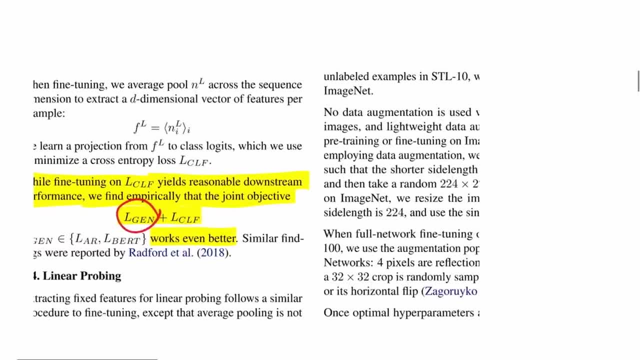 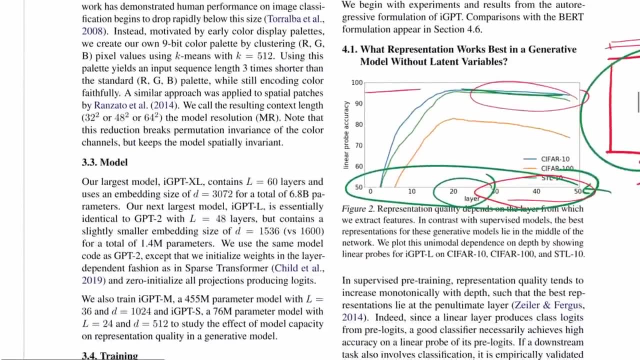 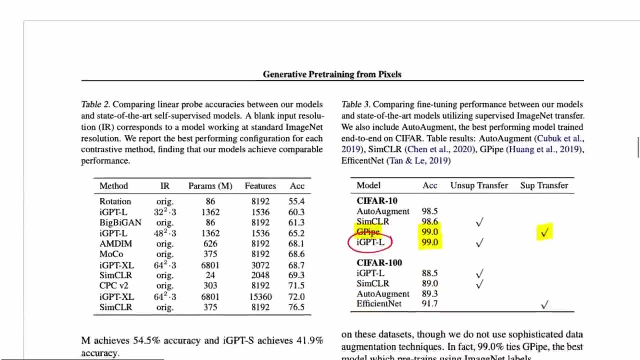 Whatever that word is. So that's also something to think about. I think this paper right here it kind of lays down a lot of cool things that you can think about and it gives rise to a lot of hypotheses of how does this stuff work? why does this stuff work? 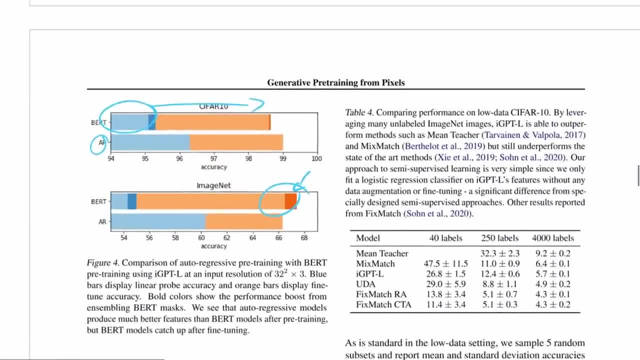 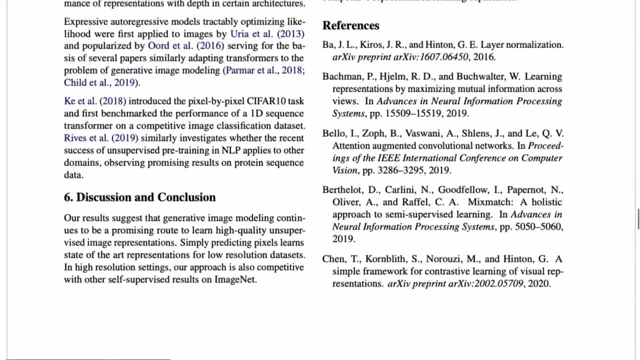 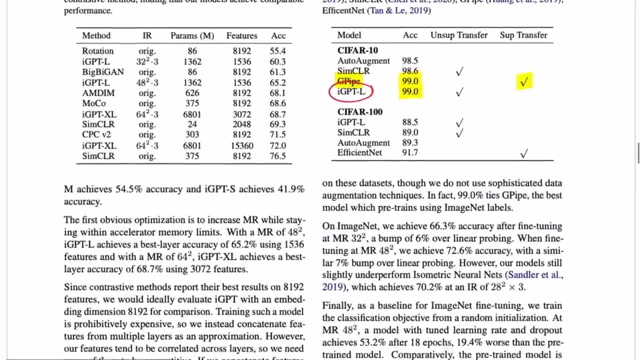 I don't even think that the numbers are the most important thing. It's mostly the fact of the effects. and what does it mean? Okay, so this was my take on it. It's more kind of my rant of what I find special about this paper than about the actual paper. 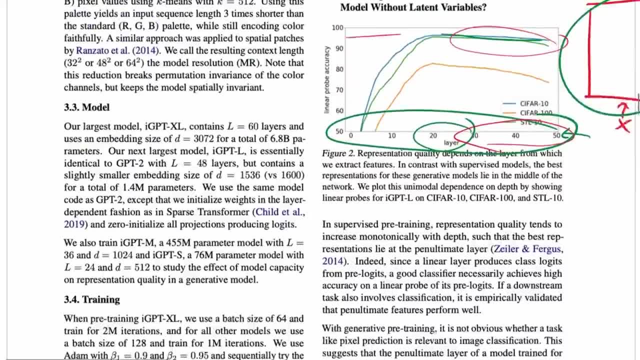 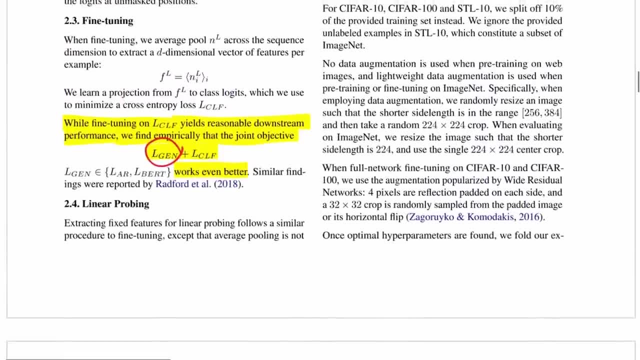 You can look at the paper. their numbers are pretty good On ImageNet. they do not reach the same like super duper performance as they do on C410. And I guess that's probably because they have to downscale the ImageNet images way more than they have to downscale.